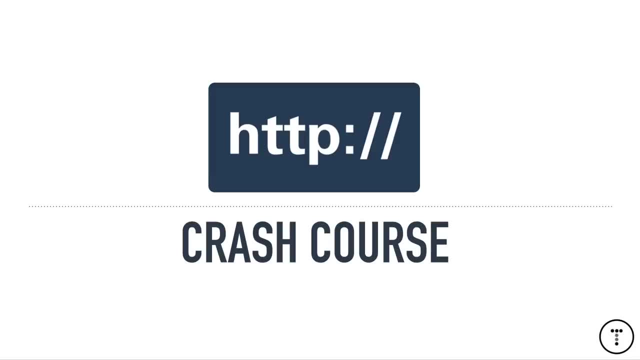 And whether you're a back-end full-stack or even front-end developer, it's important to understand HTTP and the whole request-response cycle. So in this video we're going to touch on how all this works. We'll look at the different types of responses: methods, status codes. 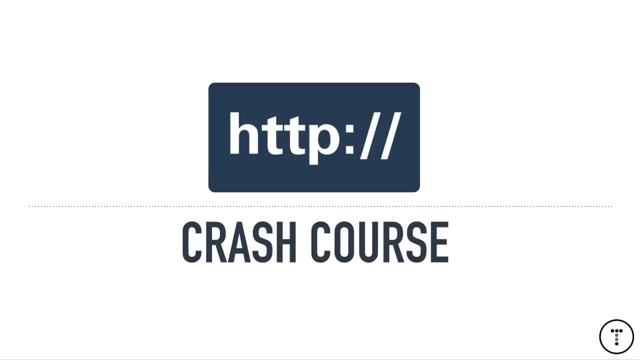 and what you get back from a server when you send a request, And we're going to go through some slides and I'd like to test some of this stuff out with Nodejs and Express, along with Postman, which is an HTTP client, And I think Express is a great framework. 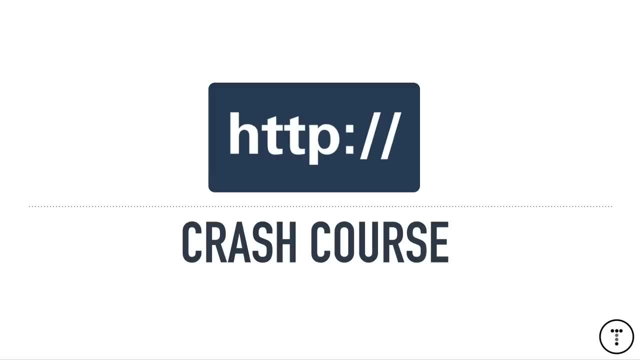 to kind of give you some examples of how HTTP works, because we handle everything ourselves. It's very minimalistic. We handle the request, the response, directly, rather than having it be abstracted like it is in many higher-level frameworks. So even if you're not familiar, 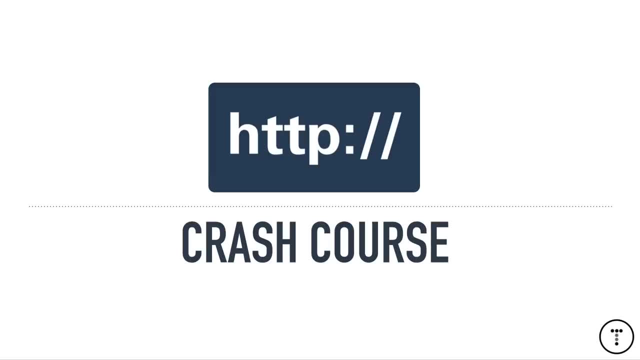 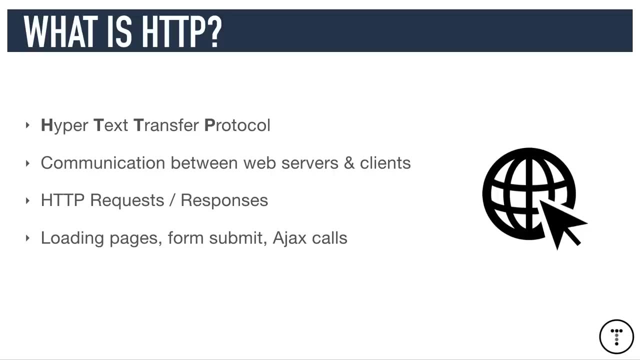 with Express or Node. that's fine. We're not focusing on the specific framework or language. So let's first talk about what HTTP is. It stands for Hypertext Transfer Protocol and it's basically responsible for communication between web servers and clients. It's the protocol of the web. So every time you open up your browser, 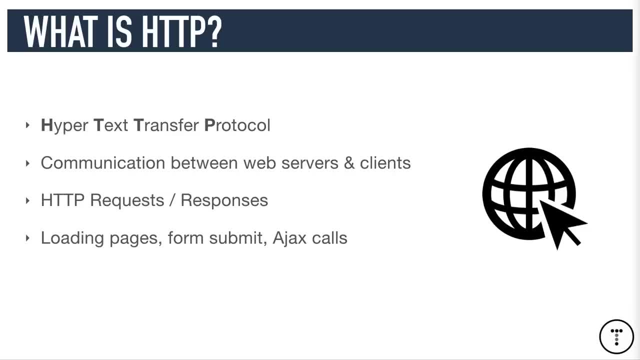 and you visit a web page or you submit a form or you click a button that sends some kind of AJAX request or fetch request, something like that. you're using HTTP and you're going through what's called the request-and-response cycle: You make a request and you get a response back. 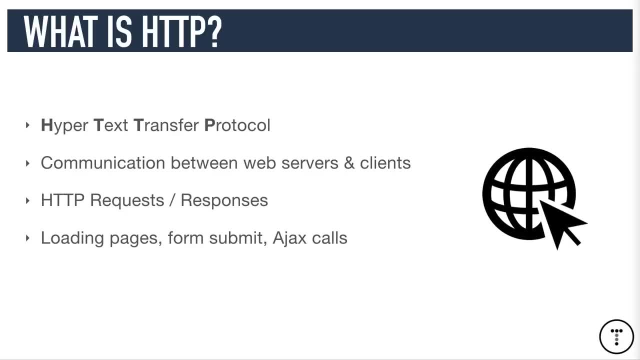 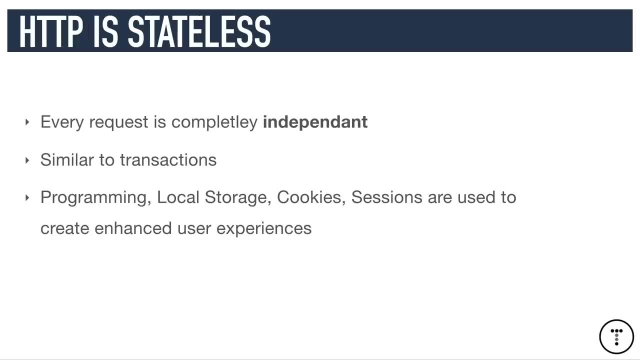 that has something called header And you're going through the request-and-response cycle And you're going to get headers and something called the body And we're going to look more into that cycle in a bit. Alright, so it's important to understand that HTTP is stateless, meaning that every request is completely. 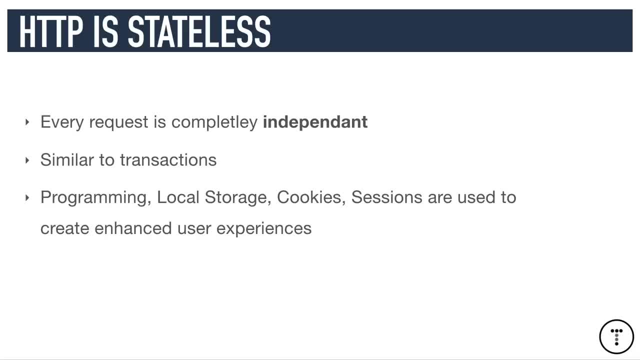 independent. When you make one request visiting a web page or you go to another page after that or reload the page, it doesn't remember anything about the previous- basically- transaction. You can kind of look at each request as a single transaction. Now there's other things we can utilize to, for instance, hold login. 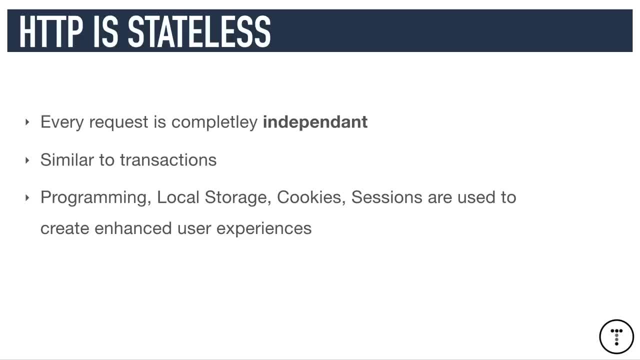 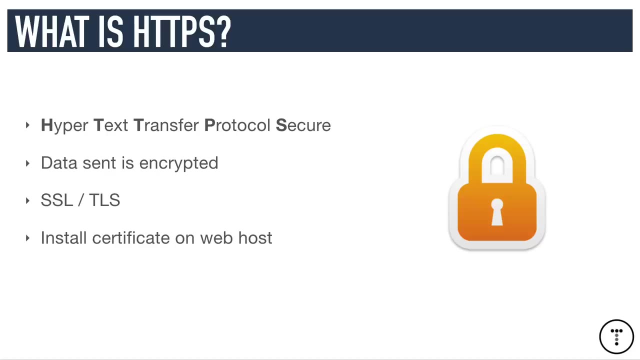 data and make a more enhanced user experience, things like programming, local storage, cookies, sessions, stuff like that- But just know that HTTP at its core is completely stateless. So what is HTTPS? And I'm sure that a lot of you guys know this stuff, but just for people that. 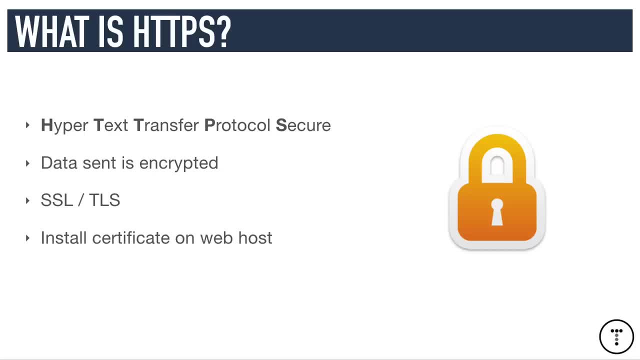 don't? HTTPS stands for Hypertext Transfer Protocol Secure, And it's basically where all the data that's sent back and forth is encrypted by something called SSL, which stands for Secure Sockets Layer, or by TLS, which is the Transport Security Layer. So anytime you have users that 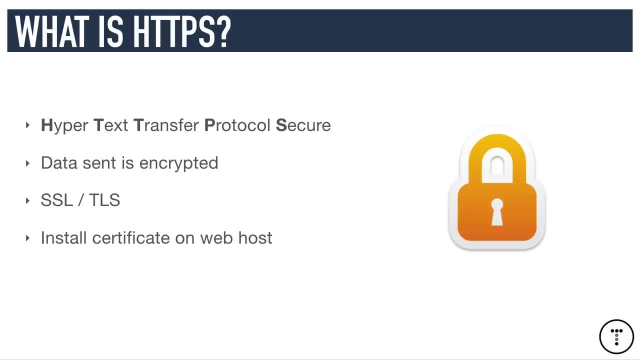 are sending sensitive information, it should always be over HTTPS, especially if it's like credit card data, social security numbers. you want to have a high level of security for that stuff And even things like contact forms. you should have HTTPS. A lot of websites and 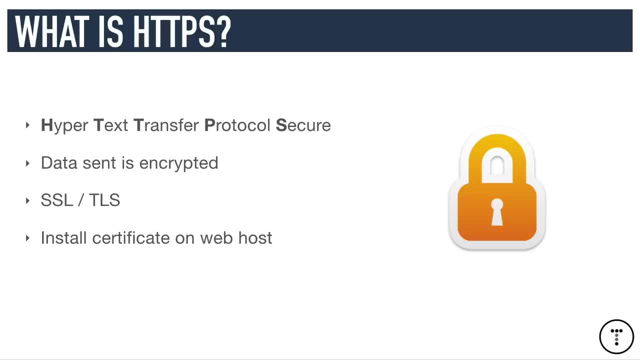 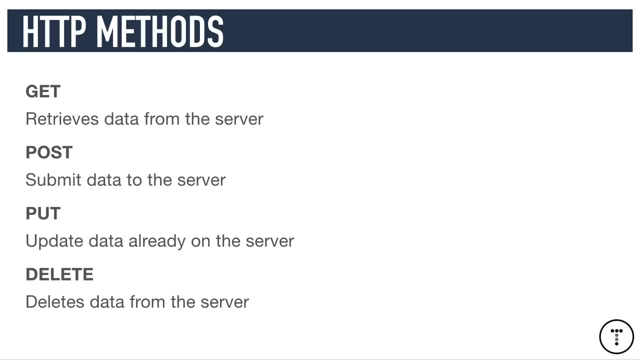 applications now are just forcing HTTPS on every page, which isn't a bad idea, And you can do this by installing an SSL certificate on your web host, And there's different levels of security, different levels of certificates as well. All right, so when a request is made to a server, it has some kind. 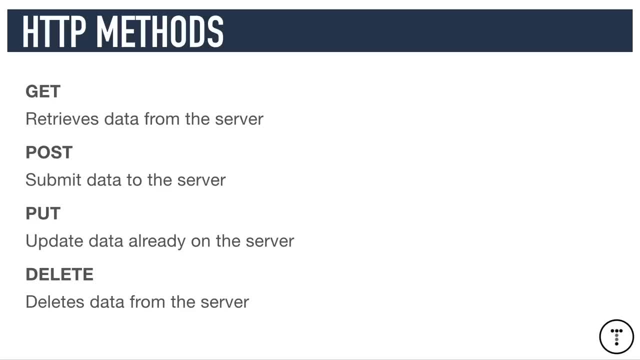 of method attached to it, And there's more than this. These are the main four that you're going to be working with And these are the ones I'm going to go over, But just know there are a couple more. So a get request is a method that you can use to get a request to a server, And you can 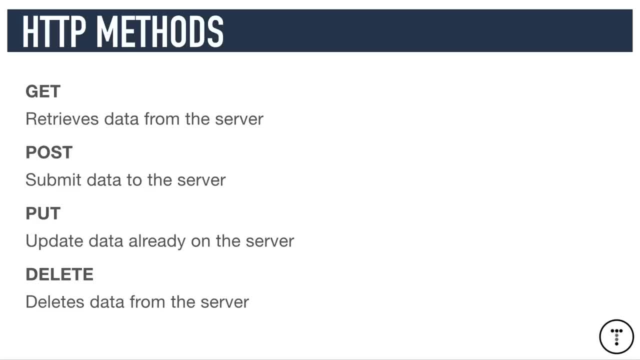 use this to get a request to a server. So a get request is used when you want to get or fetch data from the server. This could be just loading a standard HTML page, loading assets like CSS or images, JSON data, XML data and so on. So every time you visit a web page, you're making a get. 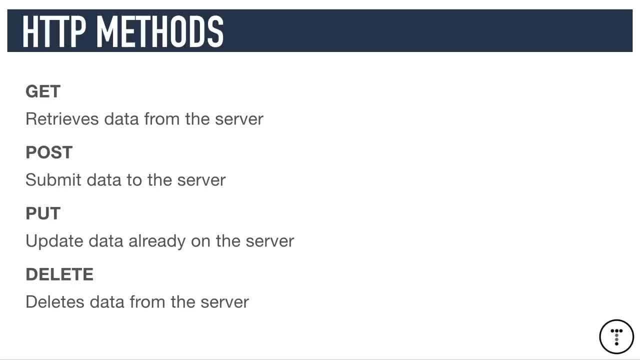 request to the server via HTTP. Now, a post request is usually used when you're posting data, when you're adding something to the server, adding a resource. Typically, when you submit a form, like, let's say, a contact form, you'll be making a post request to a server And you can do this. 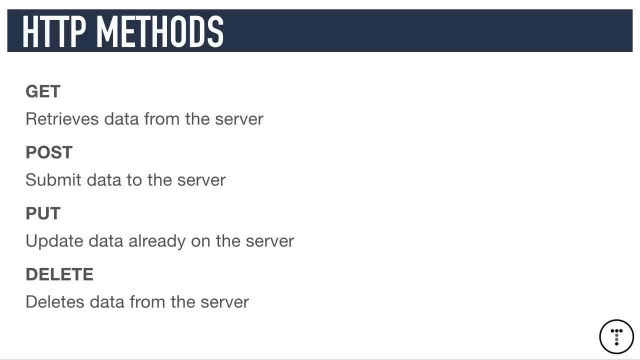 with a post request. If you're submitting, maybe, a blog post, you're creating a new blog post, that's going to be a post request. You're sending data to the server And typically that data will be stored in a database somewhere. You can also have forms that make get requests, But it's less secure. 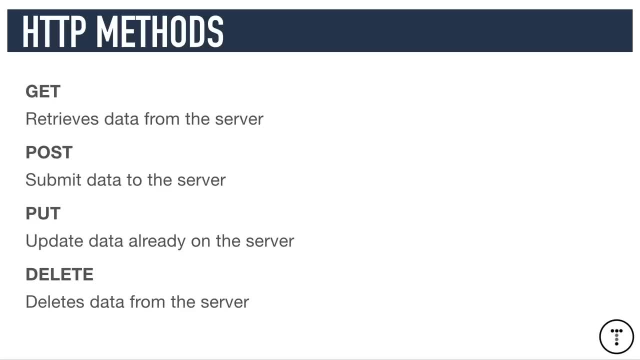 because the stuff that you send in the form is actually going to be visible in the URL. So typically you don't want to use a get request with a form, unless it's some kind of search form where all you're doing is filtering data that's coming back from the server. You're not going to. 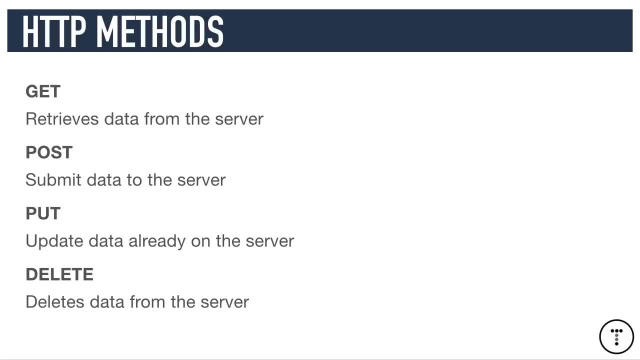 actually posting anything, All right. And then we have a put request, which is used to update data that's already on the server. So if you have a blog post, you want to edit it, maybe change the image or change some text, Typically you would do that with a put request And then a delete request. 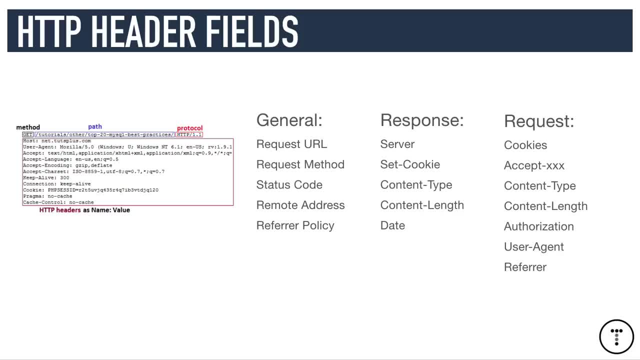 of course, just deletes data from the server. All right, So with each request and response using HTTP, you have something called a header, You have something called a body. So the body, typically with a response, is going to be the HTML page that you're trying to load, the JSON data, whatever is being sent from the server. 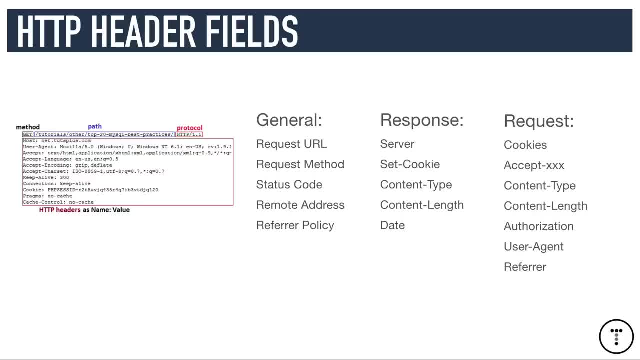 And then, when you make a request, you can also send a request body. For instance, when you submit a form, the form fields you're submitting are part of the request body. All right, Now, when it comes to the header, you also have request headers and response headers. 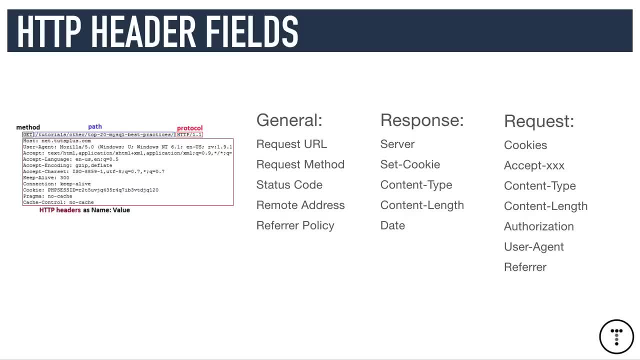 and something called a general header. OK, So it's basically divided into three parts and there's different fields on each part. So typically a header will look something like this: You'll make a method like a get request to a path or URL with a protocol. 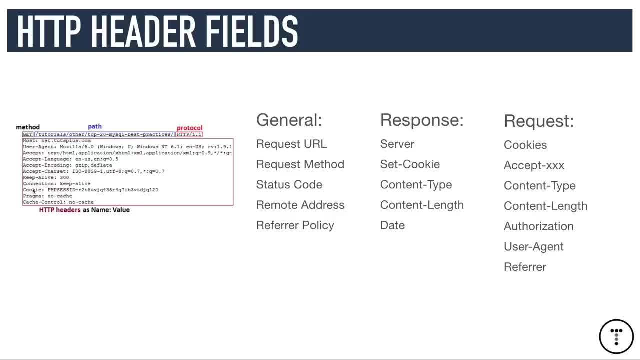 in this case HTTP 1.1.. And then you'll have all these different header fields And a lot of these you're not really going to need to care about, but it's good to know what some of the more common ones do and what they are, especially with the general part of it. So in general, 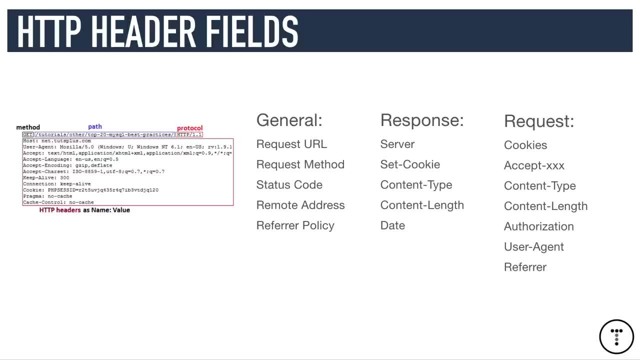 we have the request URL, which is pretty straightforward. It's just the URL you're requesting, the request method. So if it's a get request, you're going to have a request method, post request, and so on. the status code. this is probably the most important and 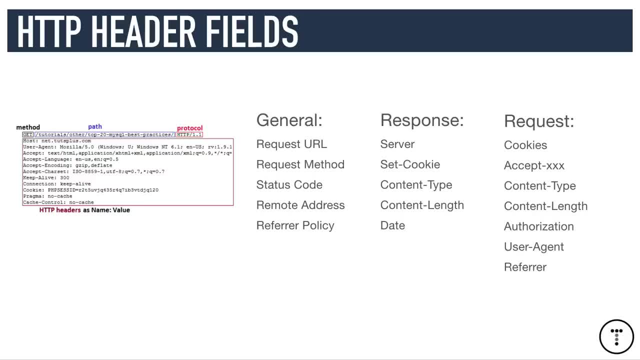 I'm gonna go over status codes in the next slide. the remote address, which is the IP of the remote computer. the refer policy: so if you're, if you go to a page from another page, it might have some information on that and whatever the Paul refer policy is, I'm not that familiar with it. the response header. 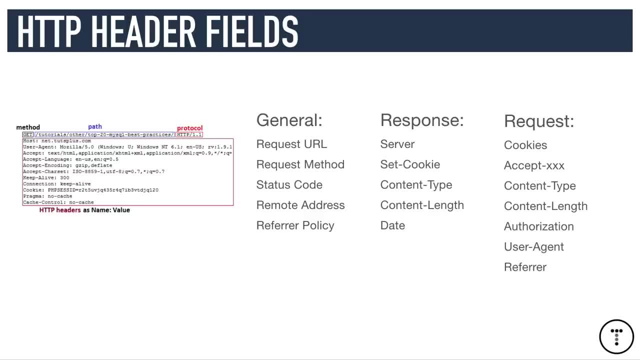 fields you have server. so if it's Apache or nginx or something like that- and a lot of times this will be hidden just to prevent hackers from knowing what type of server the, the website, uses. so set cookie is used for servers to send small pieces of data, called cookies, from the server to the client and then content. 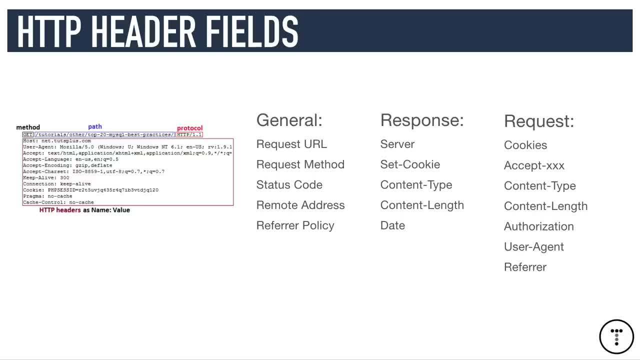 type, so every response has a content type. for instance, if it's an HTML page, it'll have a content type of text slash HTML. CSS files would be text slash CSS. images: you have image slash PNG, image slash JPEG. if it's JSON data, it'll be application slash JSON. this is 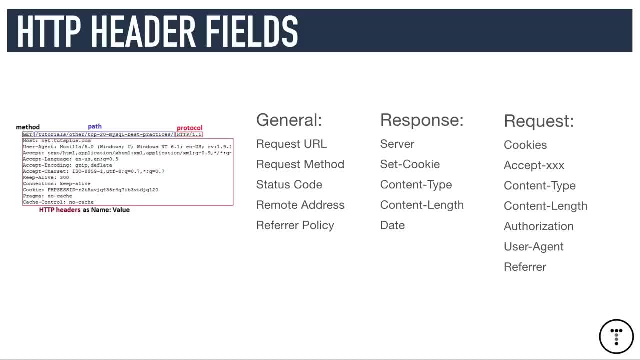 something that I think is really important to know, with the different content types. and then you also have the content length, which is just that. it's the length. it's in octets, which are, I believe, 8-bit bytes, and then also the date. okay, and there's other fields as well, but I'm not gonna list every single. 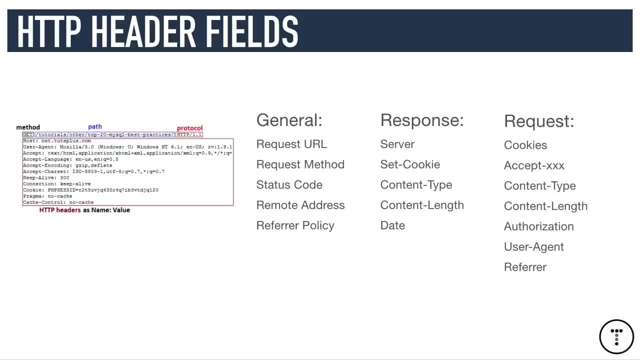 one or every possible one. so some common request fields are cookies. now, if you have a cookie that was previously sent by the server and you need to send it back to the server, you would do it in this field. you also have a bunch of except fields like accept encoding, except character set, accept language. 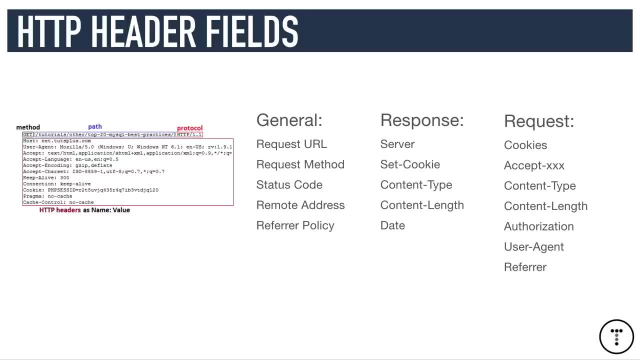 these are just the different encodings and languages and stuff that the client is able to understand. okay, Content type again. so if you're sending data, like, let's say, you're sending JSON, you'd want to set this to application slash JSON. 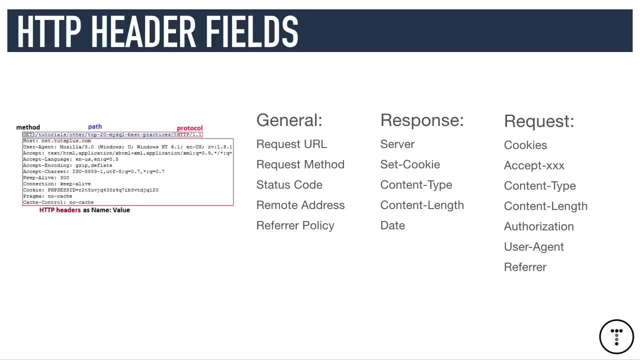 And then you also have content length as well. So authorization- remember, HTTP is stateless, so you might need to send some type of token within the header, the authorization in the header, so that you can, for instance, validate a user to access a protected route or a protected page. 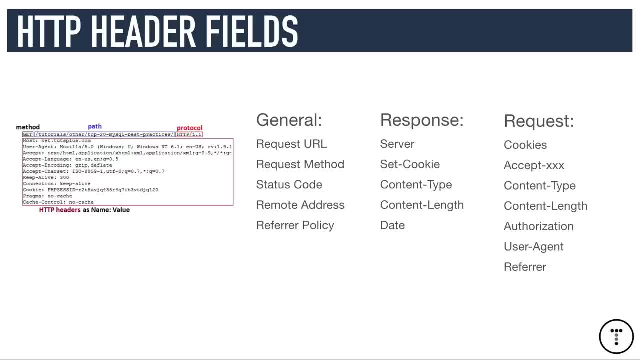 unless you're using something like sessions on the server. And then the user agent is typically a long string that has to do with the software that the user is using, so the operating system, the browser, things like that, And then the referrer has info regarding the referring site. if you were to click on a link or whatever. 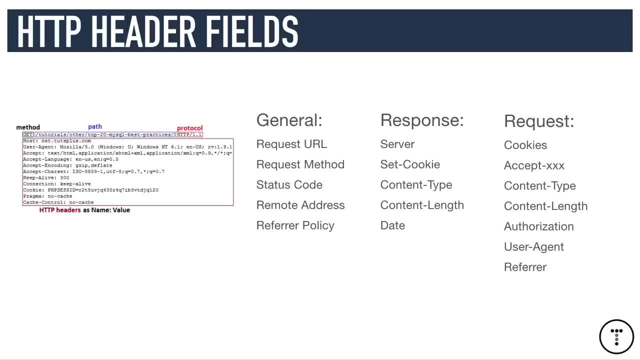 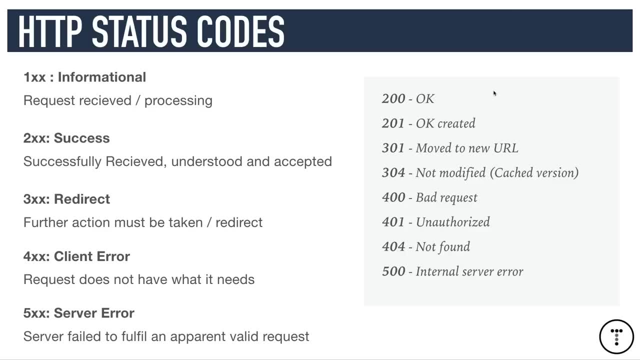 So these are just some of the more common header fields, but there are more so if you want to check out the HTTP spec, you can look more, All right. so HTTP status codes are really important to understand, at least the most common ones. 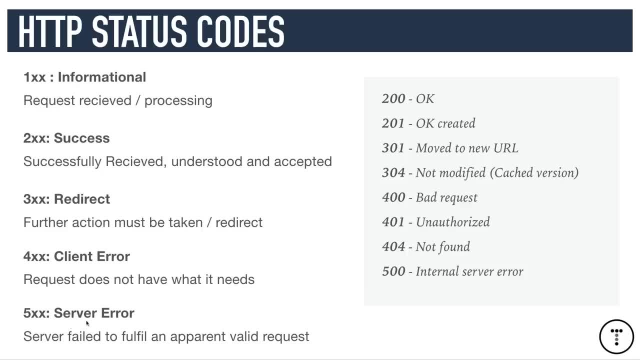 So basically you have ranges. you have the 100 through 500 range, So 100 is informational. basically, this is: it means the request has been received and the process is continuing, it's processing. 200 means that it was successful. so successfully received, understood and accepted. 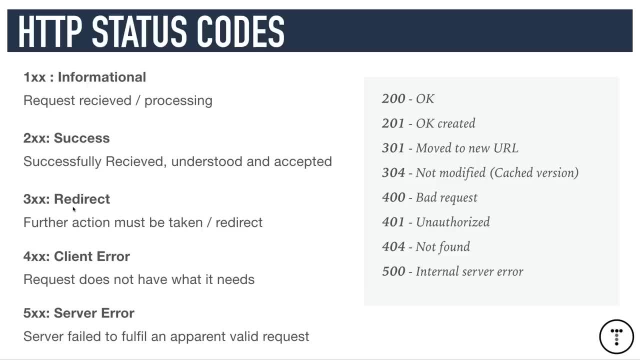 The 300 range usually has to do with research. The 400 range is a client error, meaning that the request doesn't have what it needs from the client. So let's say the server needs a name field sent in the request body and you don't send that. 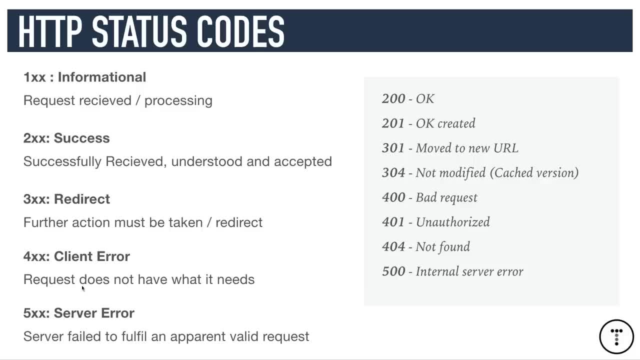 you're going to get a 400 error or somewhere in that range, And then 500 is usually a server error, so the server failed to fulfill an apparent valid request. So everything seems okay as far as what you send to the server, but you still get an error. 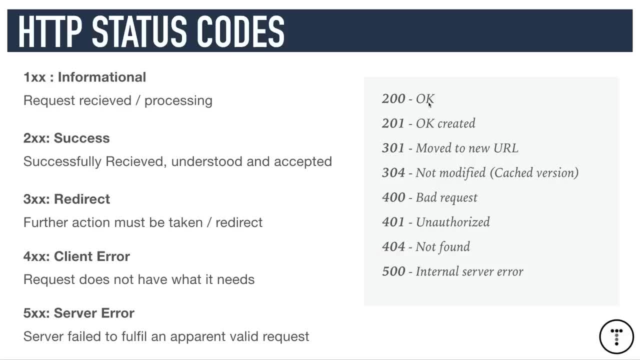 Something's wrong. Something's wrong on the server side. All right now. these are some important status codes, or I should say common status codes, that you should remember. So 200 is just okay. It means everything is fine. You make the request, you get the HTML page, you get a 200 response. 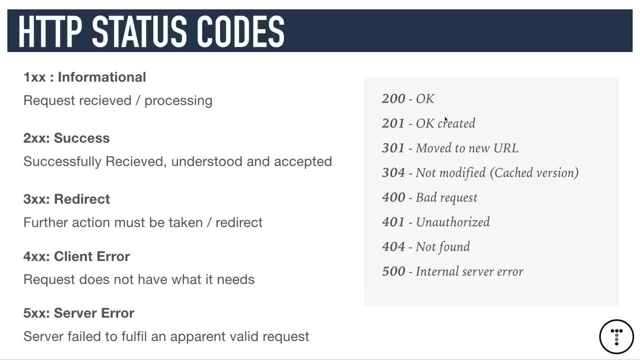 201 is okay, but it means something was created. So if you're creating a blog post and everything goes okay, then you might get a 201 response. 301 is usually moved to a new URL, So this has to do with the URL. 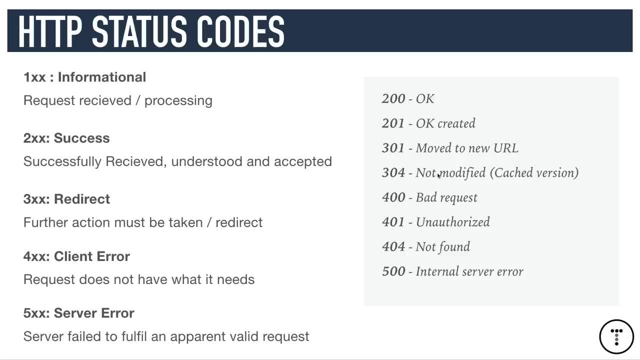 So this has to do with the URL. This has to do with redirection. 304 is typically not modified, meaning that if you visit a page and it gets cached and it hasn't changed at all, then you'll have a 304 response or status. 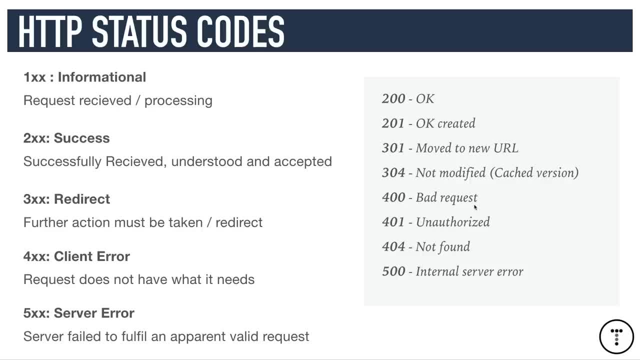 400, again, bad request. So if you're not sending the correct data to the server, 401 is typically or is unauthorized. So if you are missing a token or something like that, you're not authorized, you might get a 401.. 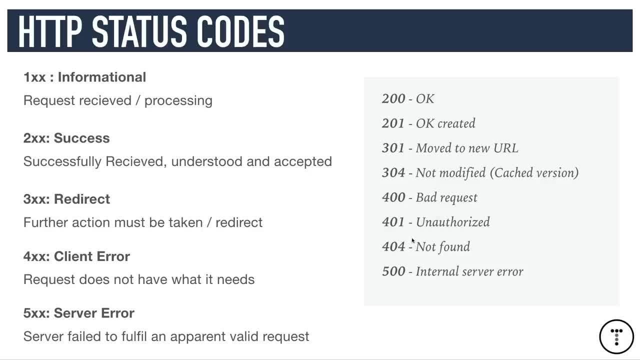 404,. we all know what that means: It's not found. If you're looking for some page on the server that doesn't exist, or some resource that doesn't exist, you're going to get a 404.. And then 500 is just an internal server error. 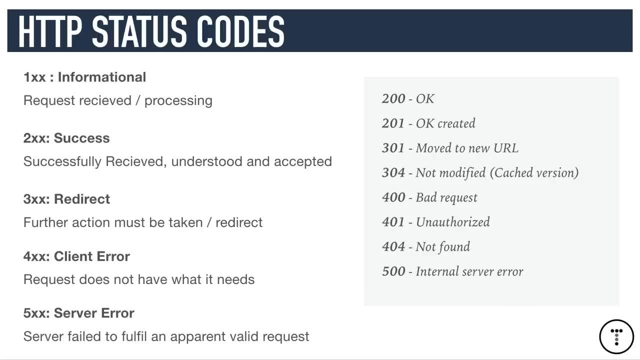 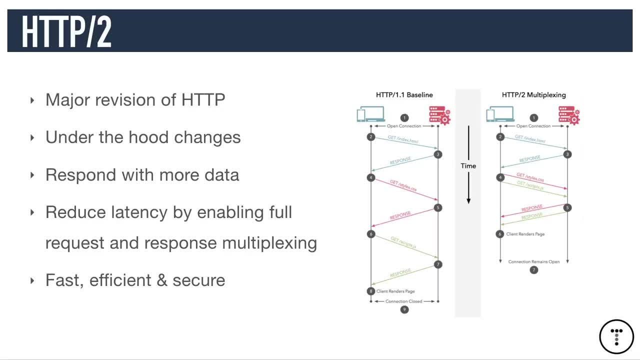 This could mean pretty much anything on the server side. All right, so those are the status codes. Those are really important to really memorize and understand. So the last thing I want to quickly mention is that there is HTTP version 2.. We've been dealing with 1.1 for a long, long time. 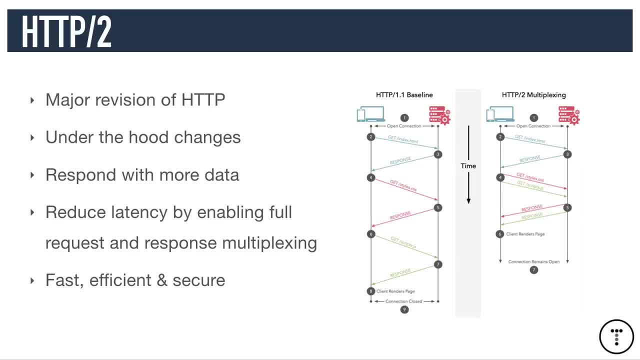 Now all the changes to version 2 are pretty much under the hood, meaning you don't have to go and change the way your applications work. All the status codes, everything like that, is all the same. It's just faster and more efficient. 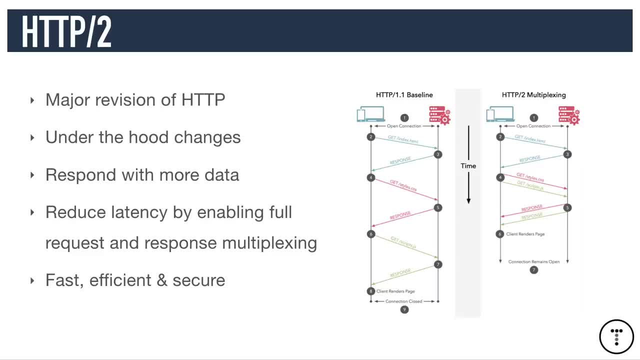 So it does stuff like reduces latency by enabling full request and response multiplexing. So it's faster, It's more efficient, It's more secure. And this is just a simple image to kind of show you that you can use multiplexing. 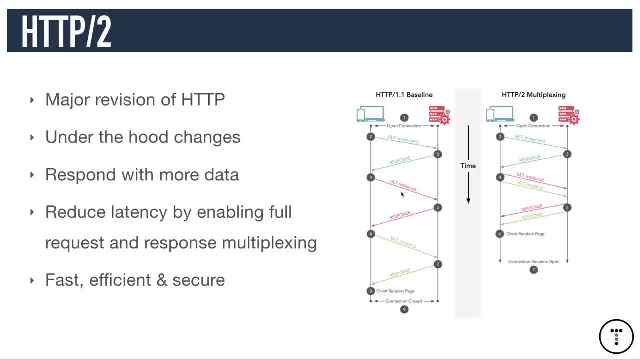 So, for instance, we get our HTML page, get a response. get our style sheet, get our response. get our script, get our response. So this is 1.1. with HDB2 multiplexing We can get our HTML and then get all of our scripts and style sheets basically in one shot here and send the responses at the same time. 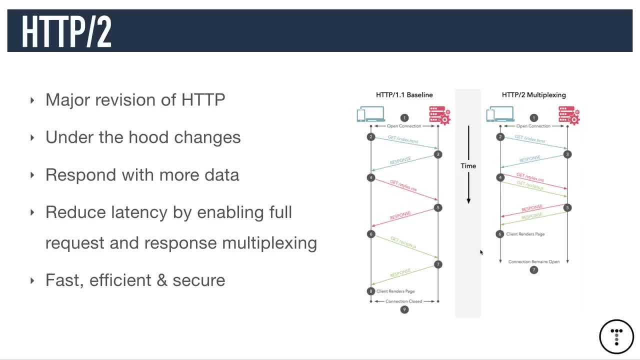 Now, I'm not extremely familiar with HDB2.. I haven't read the spec, I haven't worked with it that much, But just know it is available. It is out there, So you might want to look more into it. All right. 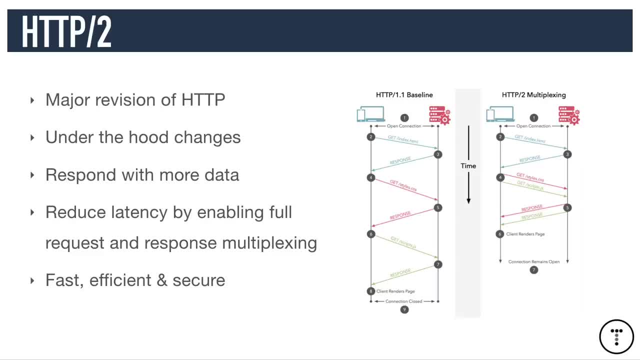 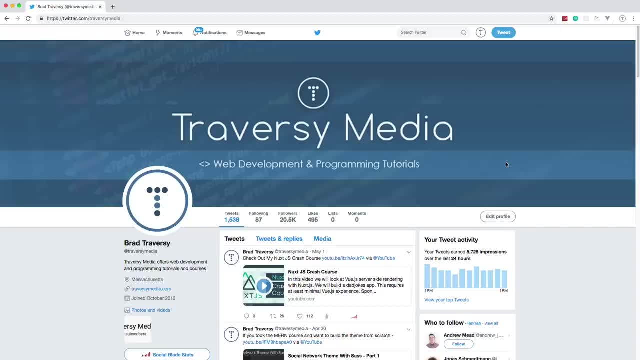 So now we're going to jump into Express so I can give you some examples on dealing with request body and headers and sending status codes and stuff like that. All right guys, So we're going to jump into our little Express server in a second. 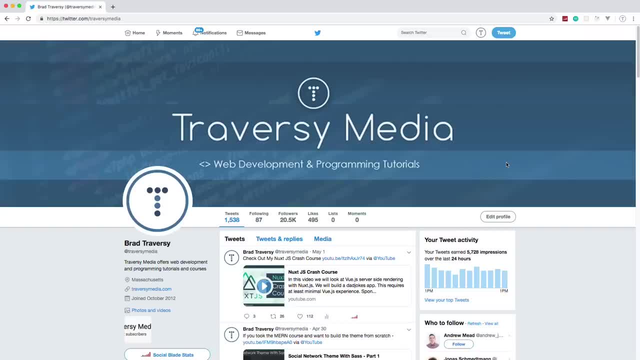 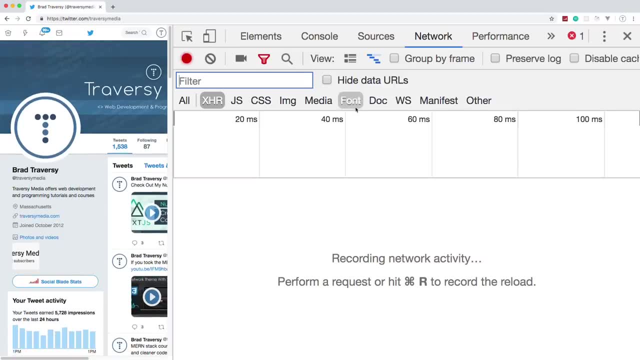 But I just want to first show you an example on an actual website. I'm just going to use my Twitter profile, But you can go to any website you want and go to your dev tools- in my case my Chrome dev tools- and then click on the network. 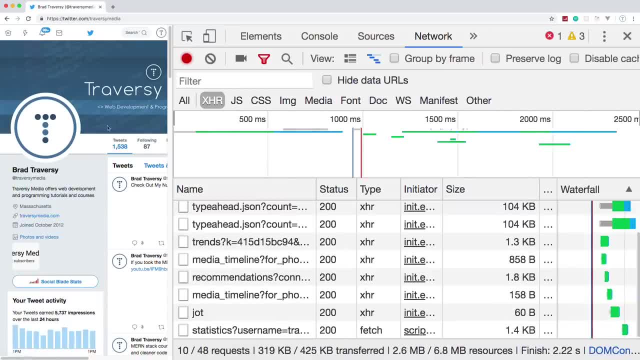 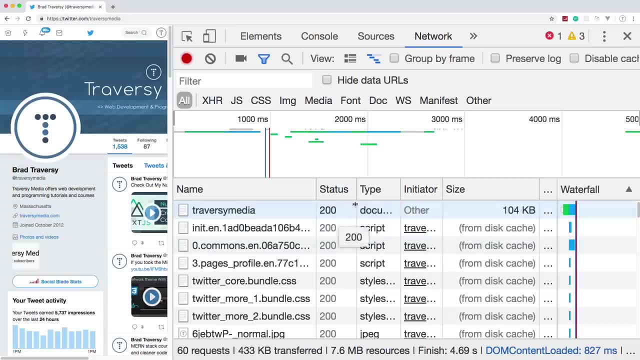 And if I go ahead and reload the page here, it's going to make all the requests it needs, it's going to get all the files from the server and it's going to show them down here So you can see the different types. the status of 200,, which means everything's okay. the size: 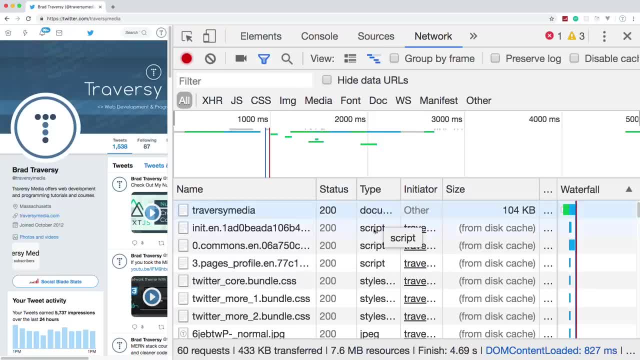 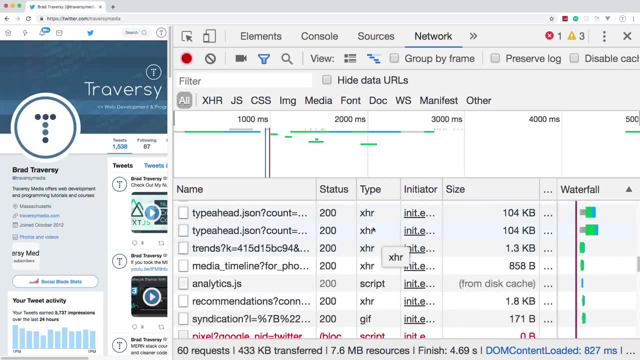 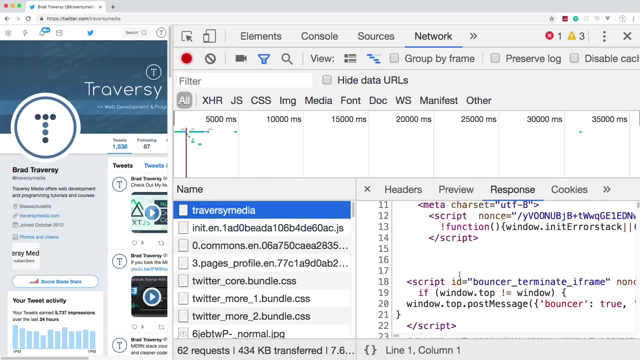 This is the document, the main HTML document, and then we have all of our JavaScript files, our style sheets, our images, XHR, which is any Ajax requests that were made. But let's take a look at the main document And, under response, you're going to see the body, which is, of course, the HTML file. 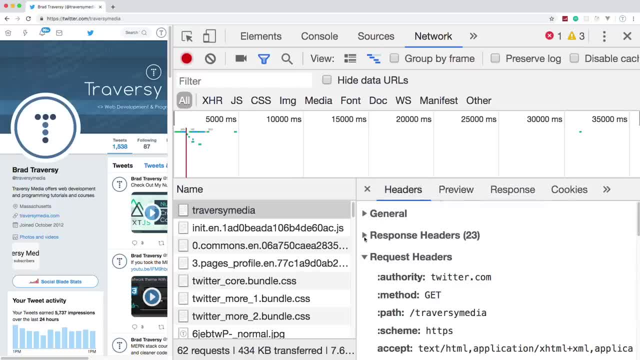 Same thing with preview. Now headers is where you can actually see all the different header fields. And remember in the slides I showed you that there's three different sections: general, response and request. So if we look at general, you can see our request URL, which is just the entire URL. 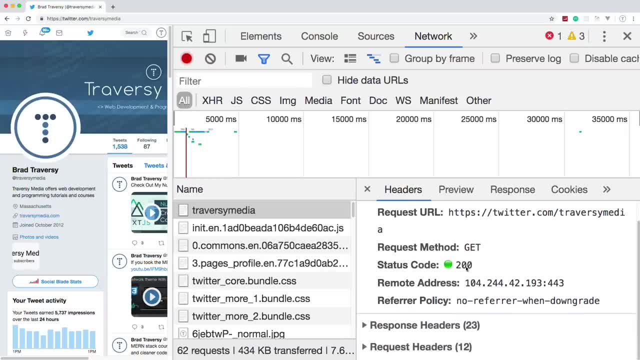 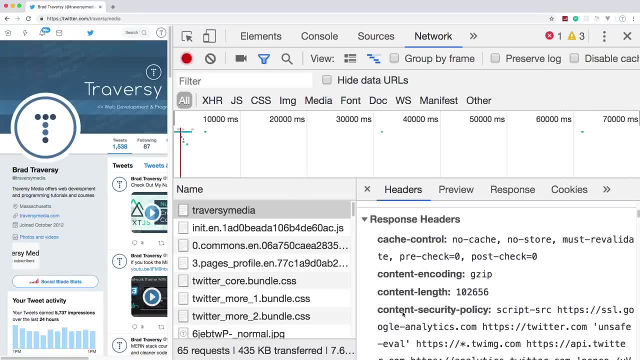 The request method is get. We made a get request. Status code is 200.. So everything's okay. We get a little green dot, The remote address and refer policy. Now, if we look in response, we have things like cache control. 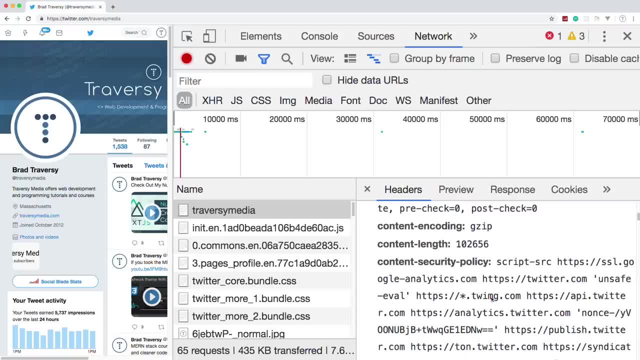 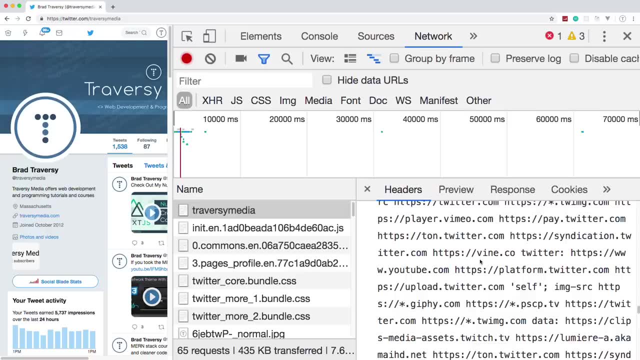 There's a bunch of stuff here that I'm not going to explain. Some of this stuff I don't even understand. But we have like the content length, their security policy, And then down here we should have like the content type, which is text HTML. 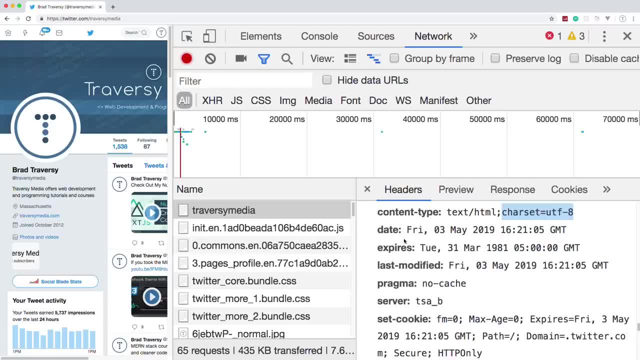 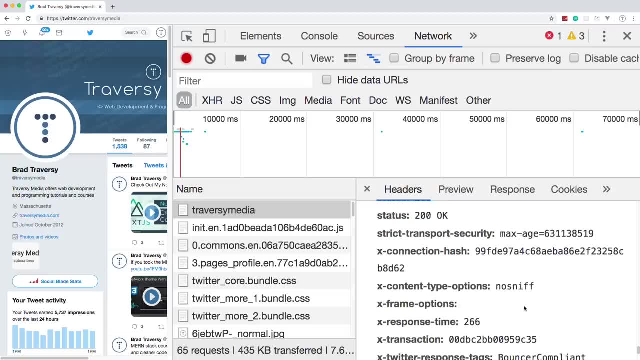 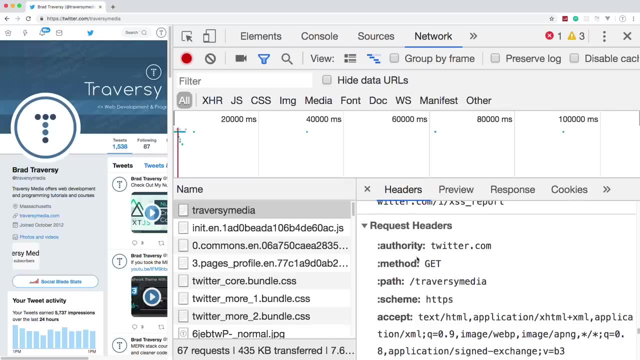 The character set is UTF-8.. The date: what else? here We have set cookie, So they set some cookies on the client Status 200 down here We have like response time, stuff like that, And then in the request headers we have the authority which is the root domain. 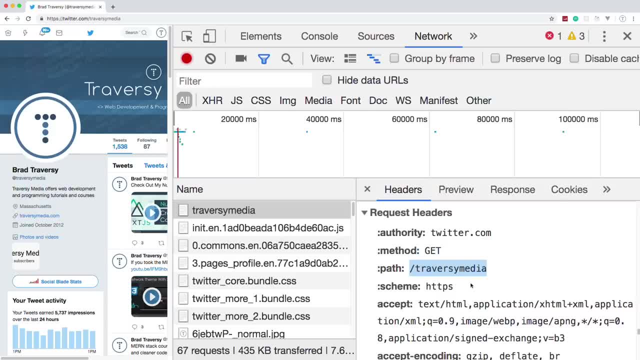 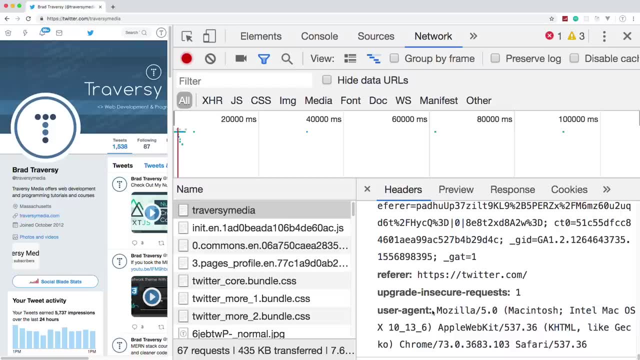 We have a. it's a get request, The path is my profile, HTTPS is the scheme, And then down here at the very bottom, we have the user agent, which is this long string which describes my environment. So it has tells you I'm on a Mac, Intel-based OSX. 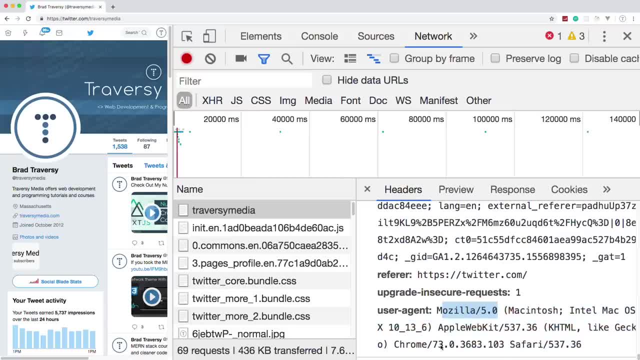 It's kind of confusing because it says Mozilla, It says Safari and Chrome. I'm actually on Chrome, so it shows the version of Chrome that I'm on. All right, so that's the user agent. So I just want you to take note of these values after what we went through in the slides. 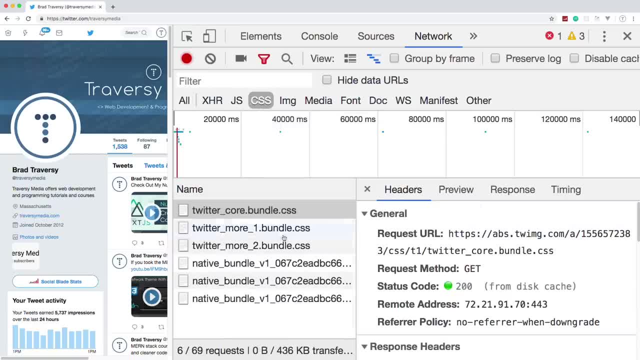 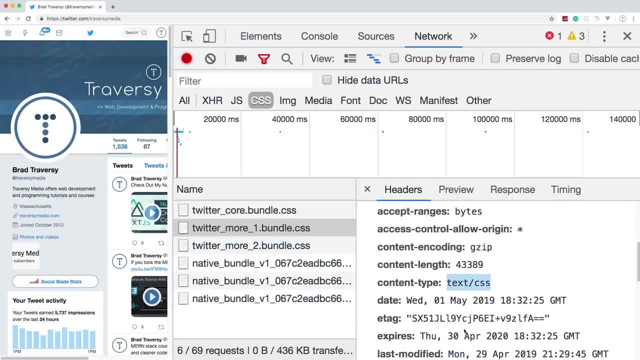 And if you want to narrow it down by files, we can see like all the CSS that was loaded. So if I click on one of these, I can see all the info for that file, including the content type, which is text CSS. 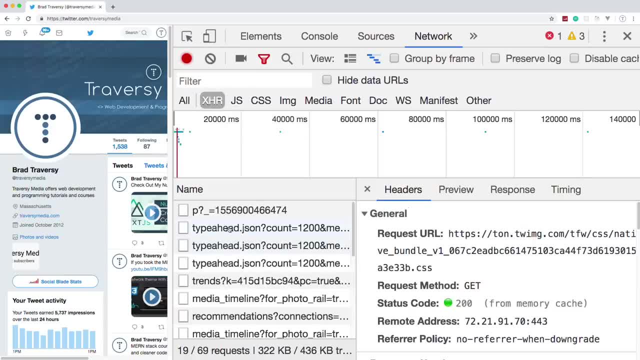 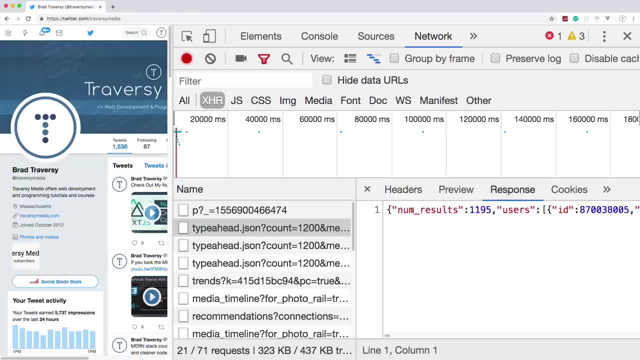 If I want to look at the AJAX request here. So like this one right here, this should be application slash JSON. And if we look at the response, this is what it got us. So the number of results, I guess some user information. 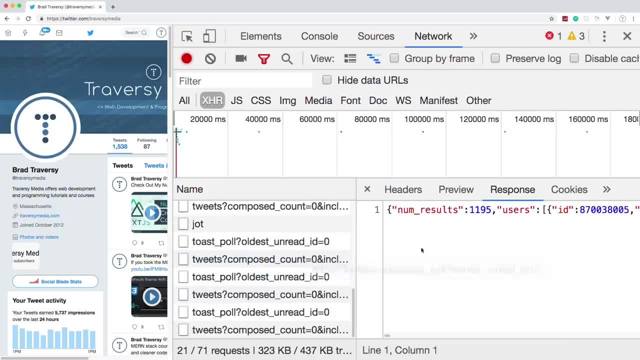 So these are all the different XHR or AJAX requests that were made. All right, so when you use the Fetch API or Axios or old school AJAX, this is where it's going to show up, So just get familiar with the network tab. 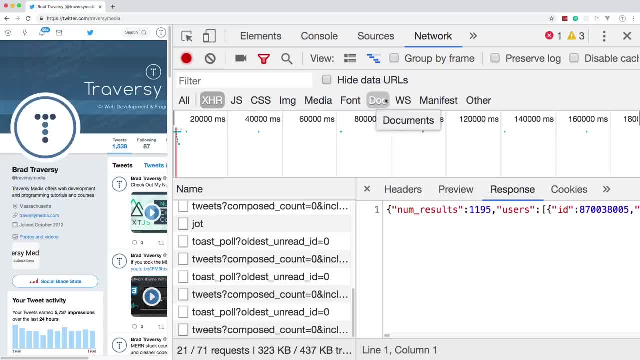 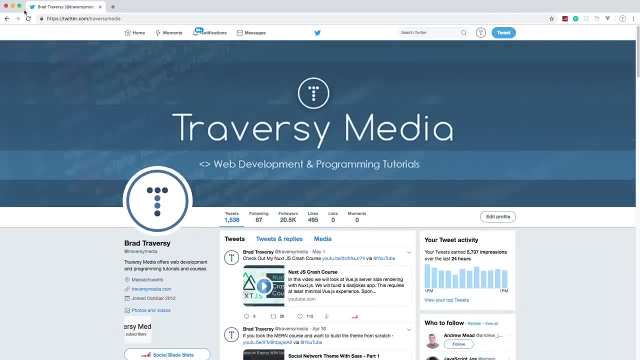 It can be a little daunting at first, But it's really helpful. It lets you know what's going on, It shows you the load times and all that stuff. All right, so enough with that, Let's jump into. I'm going to show you Postman first. 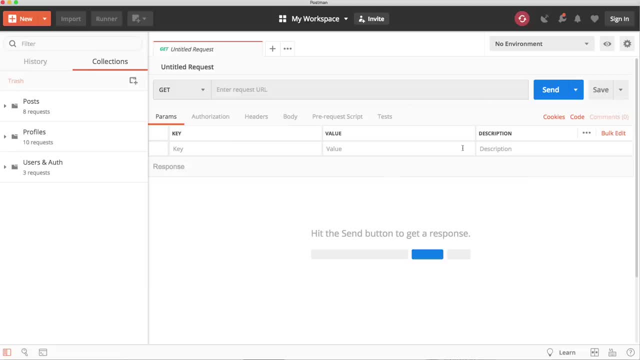 And if you don't have this client- which is just awesome, especially if you're building APIs- you can get it at getpostmancom And, as you can see, I can make any type of request. So get post, put patch, delete all these other ones- to any URL. 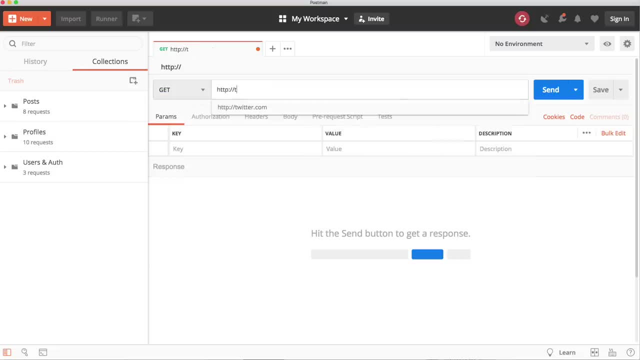 In fact, I'll go ahead and make a request. I'm going to make a request to twittercom, slash, travestymedia, slash, Okay, and I'm going to make sure it's a get request, just like the browser made, And I'm going to get the same exact thing. 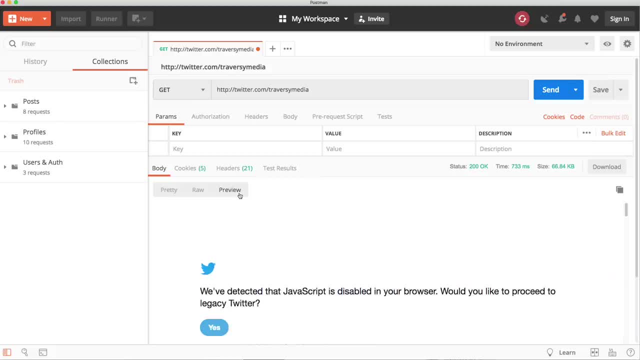 I'm going to get all the HTML. It doesn't render it. Well, actually, can we preview it? I've never actually tried to preview HTML. It's disabled. Would you like to proceed, Legacy? Yeah, so whatever, You get the HTML. 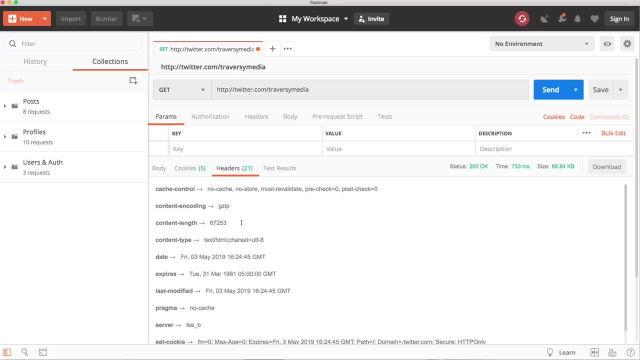 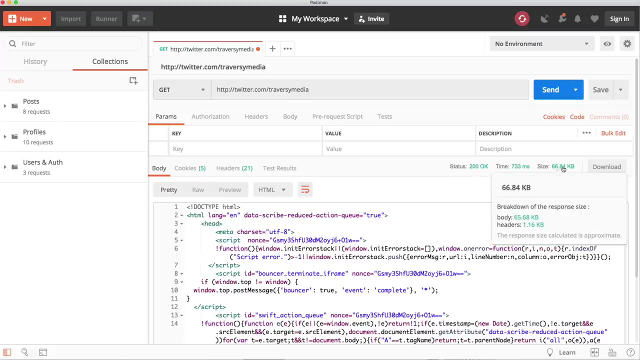 And then headers. We'll give you all the response headers so we can see the content type that we're getting set, cookie status, all that stuff. If we want to look at the cookies, we have that tab as well. It shows us the status up here as well, with the load time and the size. 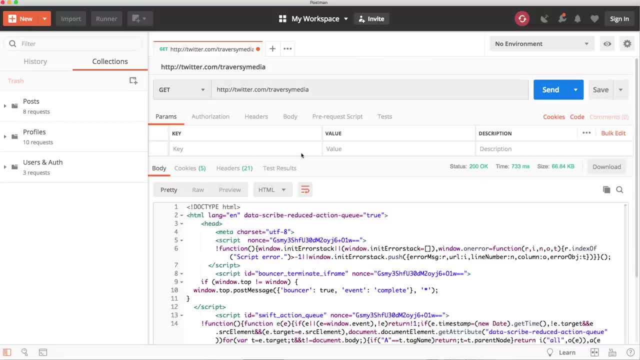 OK, so we can make any requests from here that we can make in the browser and more, because we can actually do put and delete and all that stuff. So this is a fantastic tool for testing APIs That you're building. So let's jump into express real quick. 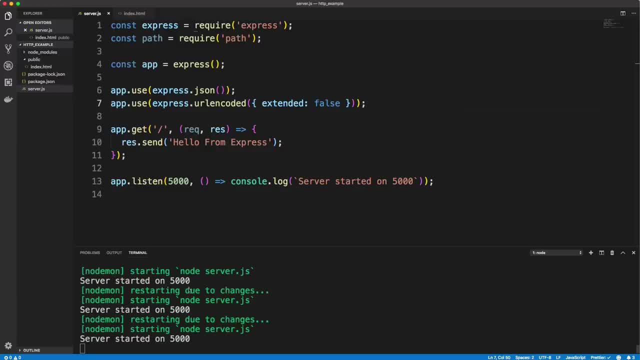 I just have a basic express server running here on local host. five thousand, and don't worry about it if you're not familiar with express. Basically, all we're doing here is bringing it in, initializing it, setting it to listen on port five thousand. 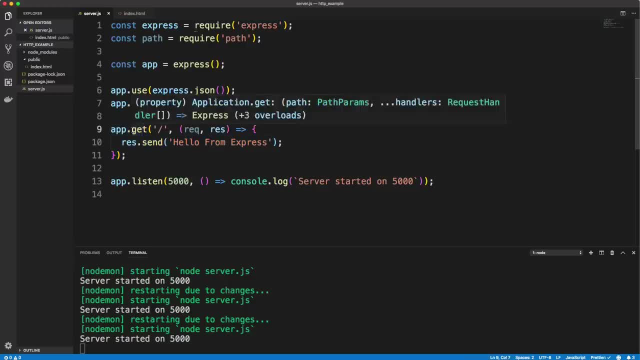 And we have one end point, meaning that if we make a get request- so we said app dot get to slash, which is the index page, It's going to run This function that has access to this request and response object And with our response object we can call dot send, which will just send, basically just whatever we put in here to the client. 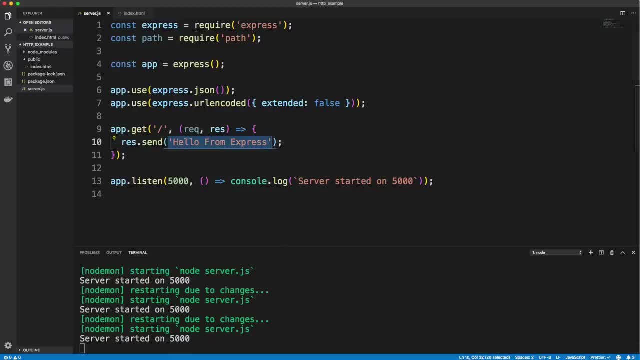 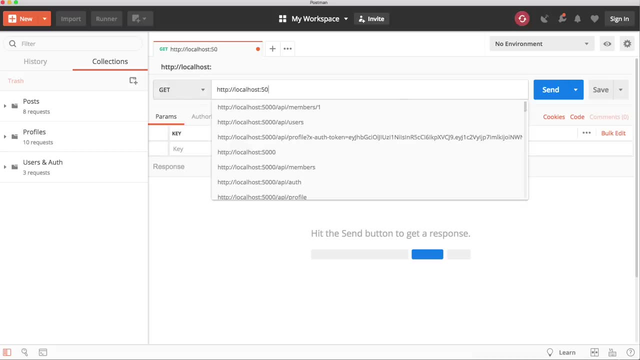 OK, in this case just a string of hello from express. So if I go to postman and I make a get request to HDP local host port five thousand, I get hello from express and I could do the same thing in the browser. 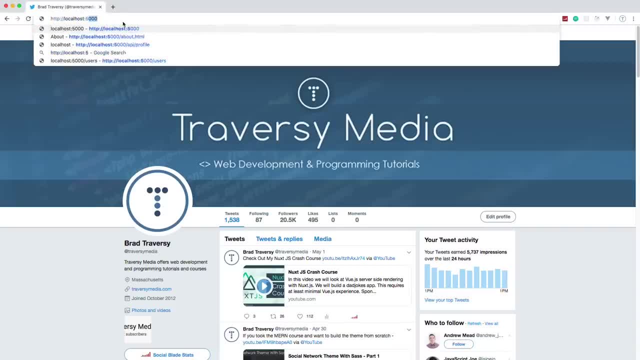 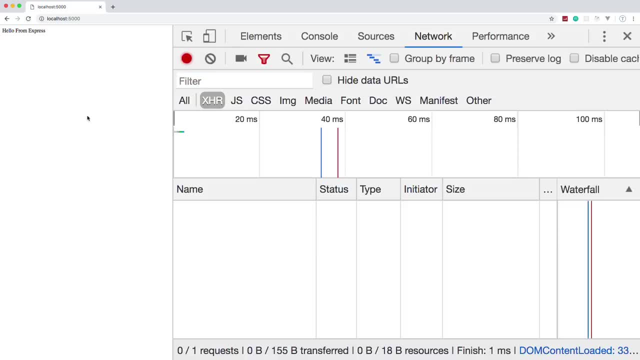 So I'm going to go to all and get hello from express. All right, If I open my network tab and reload Up, we're going to go to all here and you can see that I get a three or four, which means not modified, because it was cast and it didn't change. 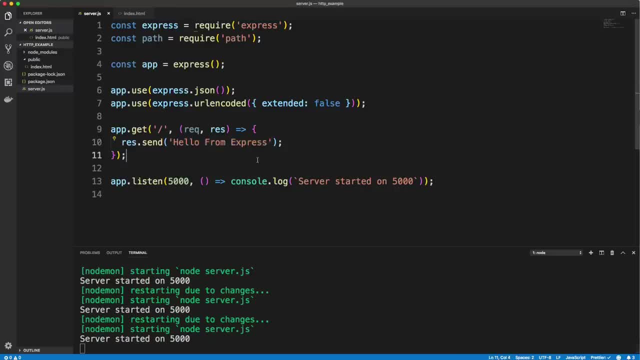 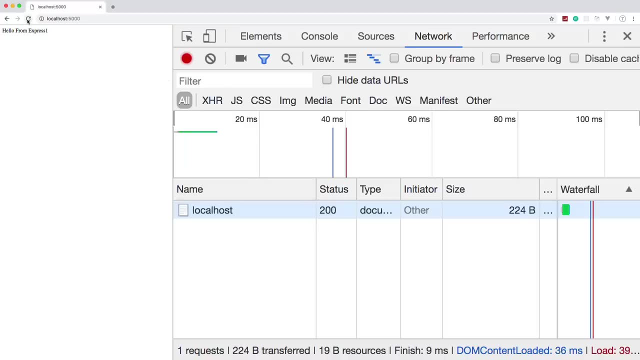 So it gave me this three or four. If I were to change this, like say hello from Express one and save and go and reload, now I get a 200.. If I reload again, I get a 304, because it didn't change, But over here. 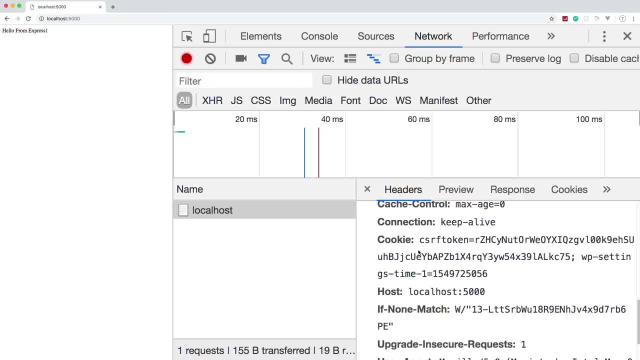 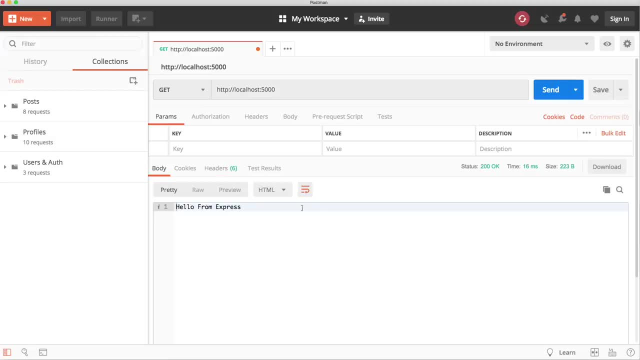 I can see all my headers. So same stuff that I saw with Twitter. there's just a lot less because there's a lot less going on, All right. so in Postman, same thing: I can see all my headers. Now, with Postman I can send all kinds of stuff. I can send a request body, I can send headers. 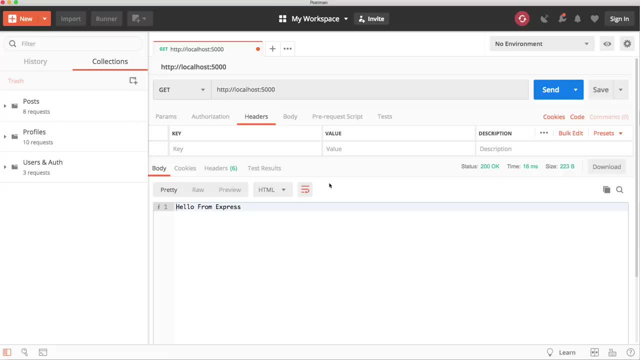 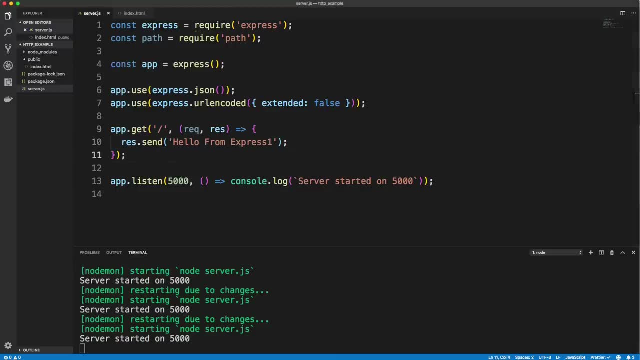 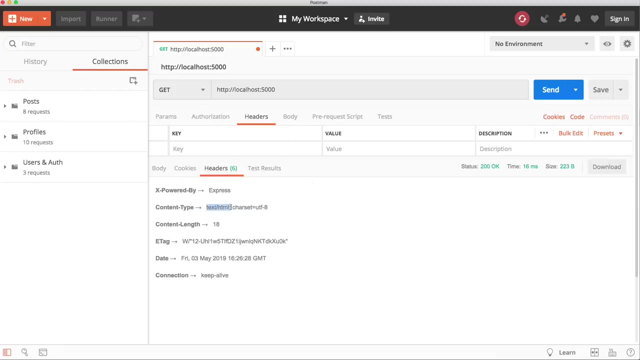 So we have a lot more freedom to basically interact with the request and response cycle Now in Express. actually, one thing I wanted to show you is the content type which, by default, if you use ressend and you just send a string, it's going to be HTML. Okay, in fact, I could. 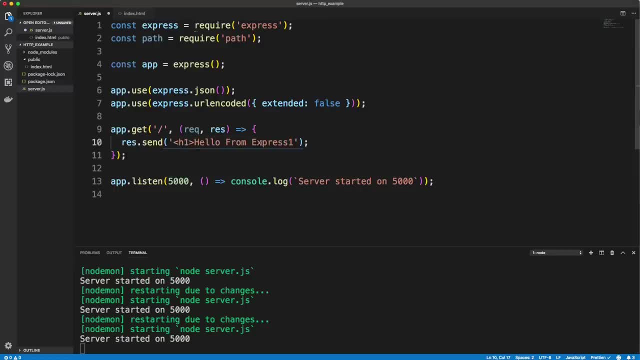 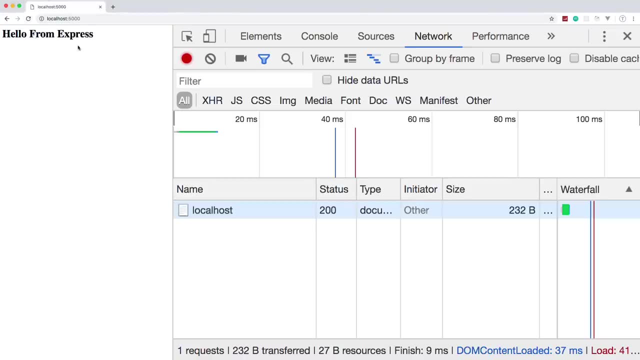 put. I don't want to make this too much about Express, but I could put HTML right in here And if I go to my browser you can see that that actually renders All right now if I were to put Jason in here. 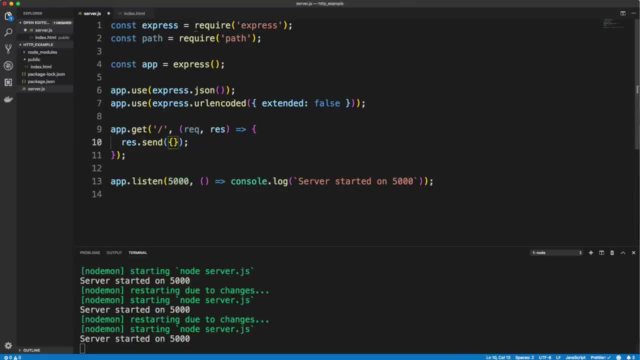 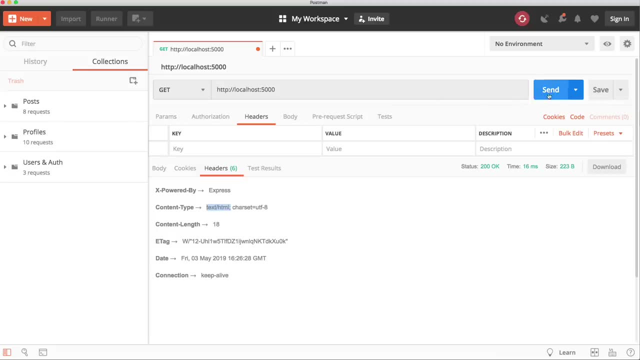 let's get rid of this And let's say MSG. we'll just say message Hello And I save that And we go back to Postman and send. you can see the content type has changed. So with Express ressend, 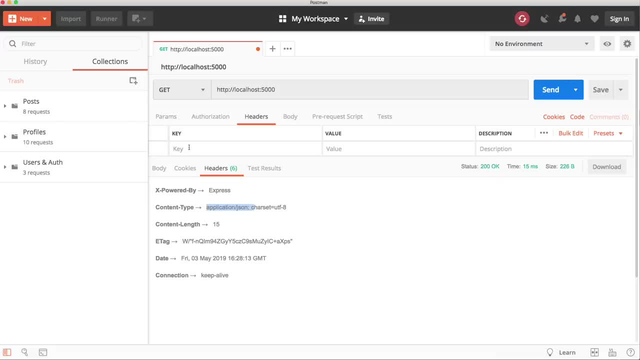 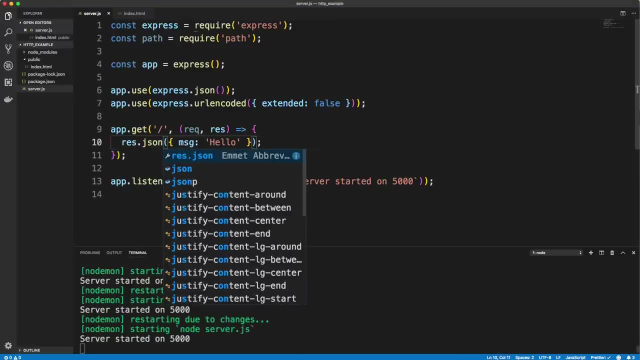 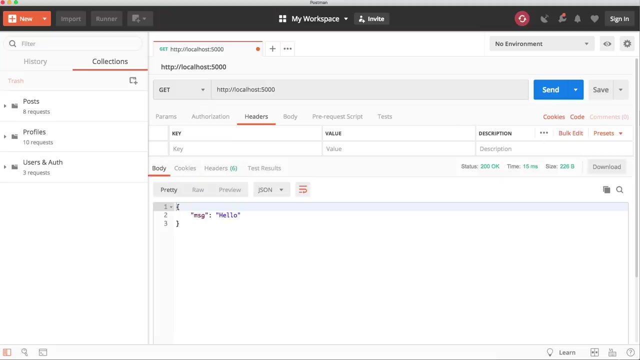 will basically detect the content type as best as it can. Okay, but there is a resjson, which is what you should use if you're sending Jason. So if I do that, it'll give me the same thing. All right, it shows the Jason in the body. Now we can also get our. 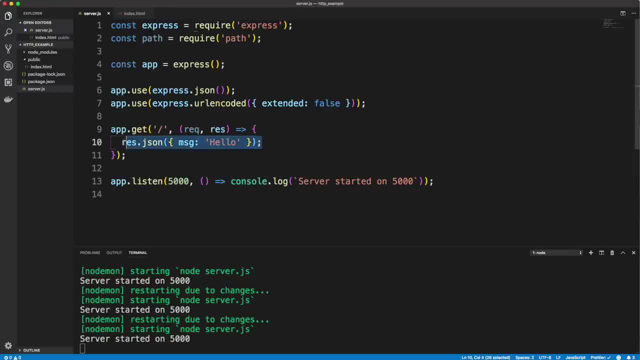 header values or header fields if we want. So I'm just going to do a ressend just to kind of show you the output of this. But if I take my request object I can do dot header and then in parentheses any header value I want, like let's say the host. So I save that and I go back to Postman and send. 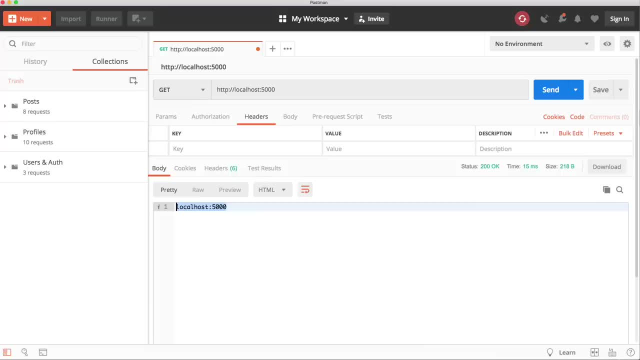 I get a response with my host, localhost 5000.. Okay, if I wanted, let's say, the user agent, we'll do user dash, dash agent And if we go back and send, we get, in this case, Postman runtime, because I'm using Postman as a client. So this is. 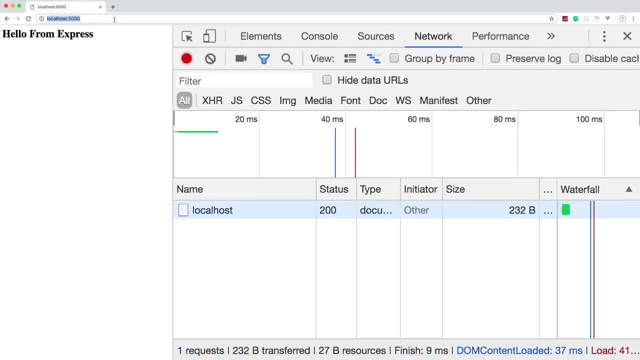 going to be different than what we saw in Chrome. If I go back to Chrome and reload, we're going to see this, okay, which is different because we're using a different utility, a different client, All right. so just wanted to show you we could do that. We can also get just the. 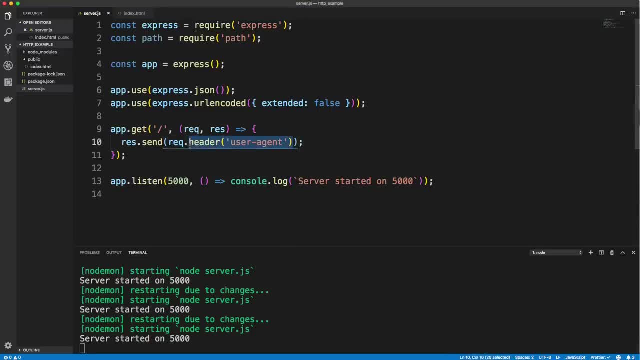 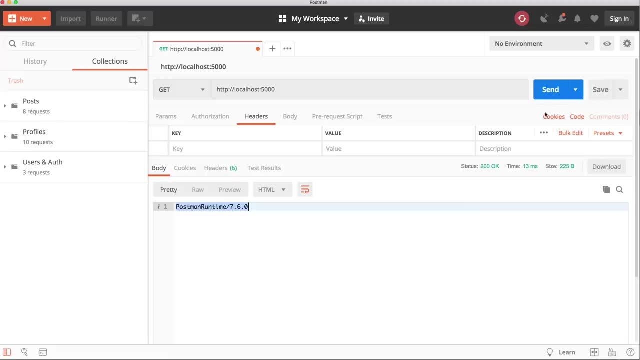 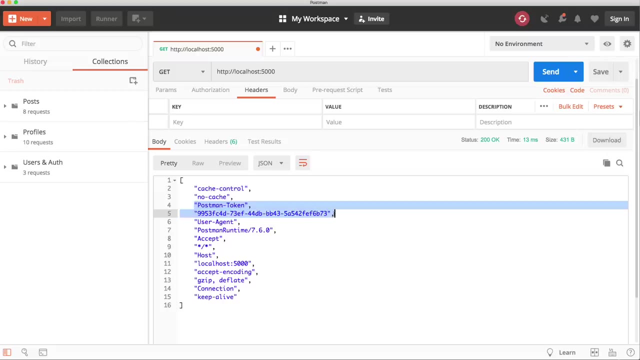 raw headers, So basically all of them. if we do request dot raw headers And if we go back to Postman and send, you can see we basically get an array with all the headers: the cache control, Postman token- since we're using Postman- the user agent, the accept value, the host, all that. 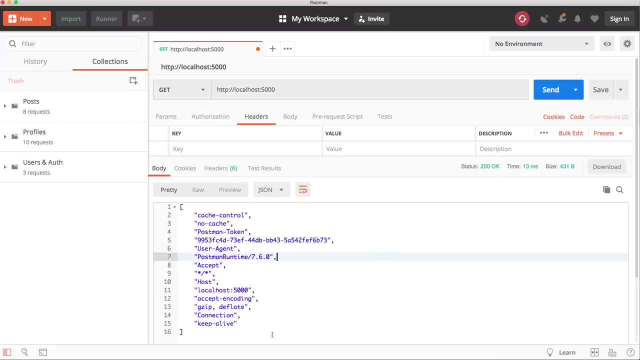 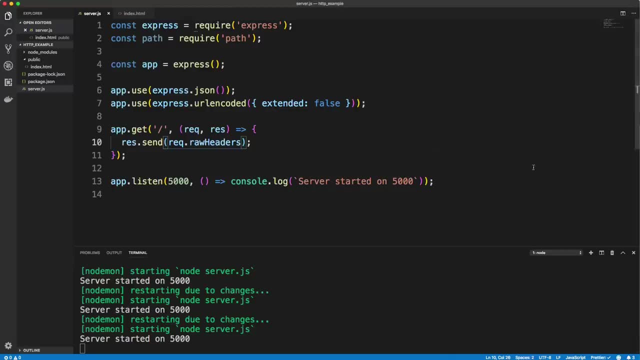 stuff. Okay, and we can send headers as well, which I'll show you in a little bit, So we can get header values. What else do I want to show you? So let's actually, let's change this to a different row, Let's do like slash contact. we'll say that this is a 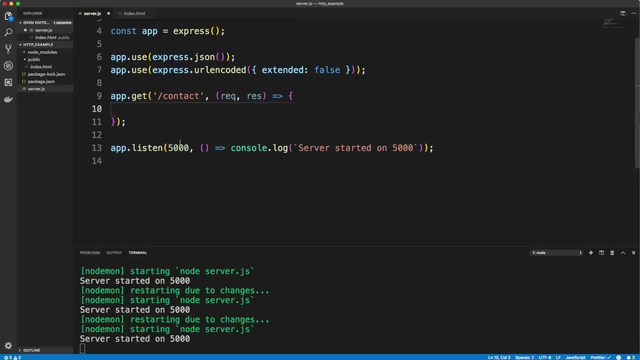 contact form, And what I want to show you now is how we can send data to the server in the request body. When we send a request, we can attach data to that, to the body And the way that we access that. I'll just go ahead and send it so we can send it to the server And then we can send it to the. 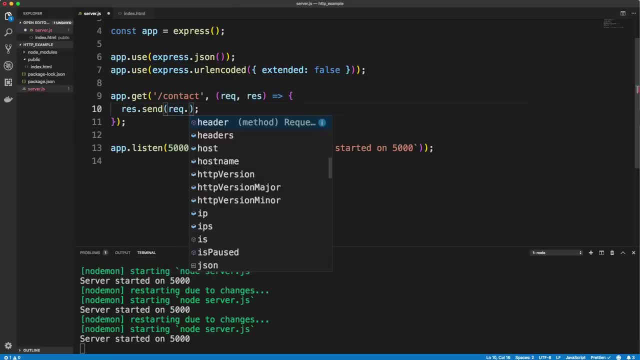 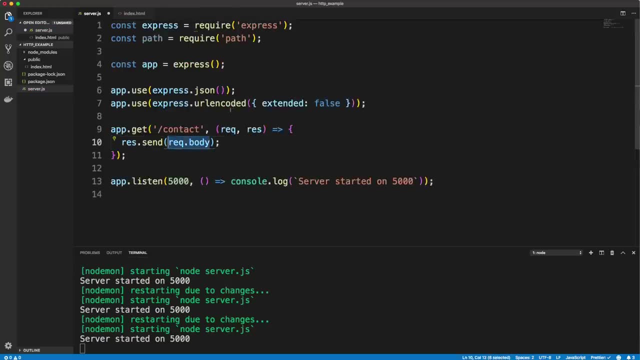 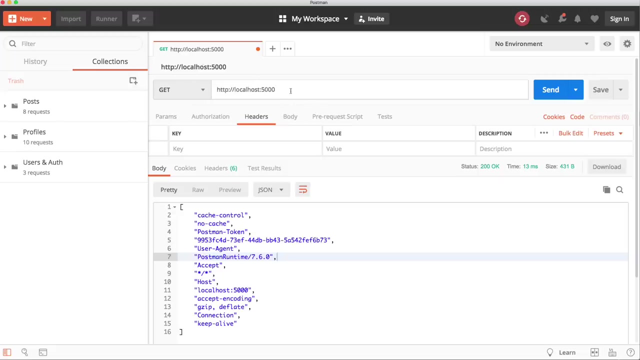 request body. Now, this won't work for for JSON data, unless you put this piece of middleware in, and it won't work for form data unless you put this in. That's just an express thing, All right, but let's go ahead and save that, Excuse me, And let's make a request here to 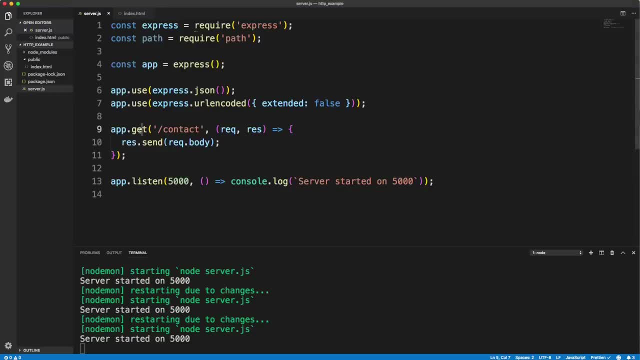 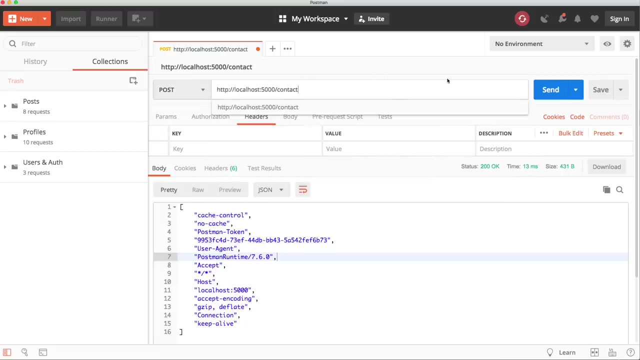 actually I want to. I'm sorry. I want to change it to a post request. Okay, if you're sending data, you want it to be a post, So we simply change: get to post here. So I'm going to save that and go back and then make a post request to slash contact Now. 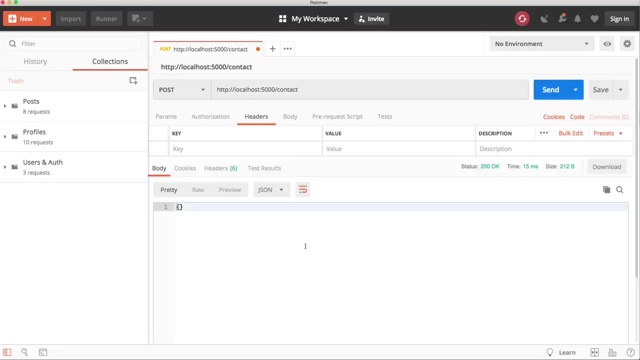 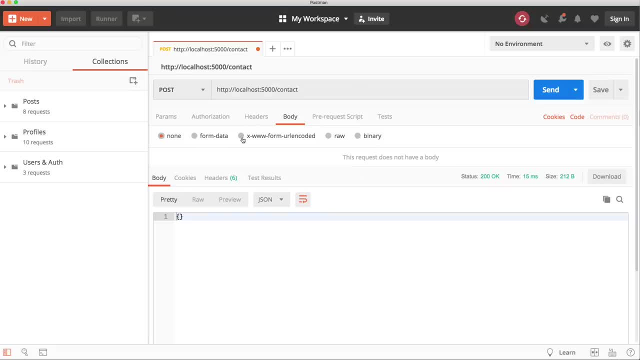 API, So from here I could send form data if I want. Now notice when I click this www form URL encoded, it automatically puts a content type in my header. Okay, because you need to send this along to. so we're actually sending a header value here, And then in the body I could put a key like let's. 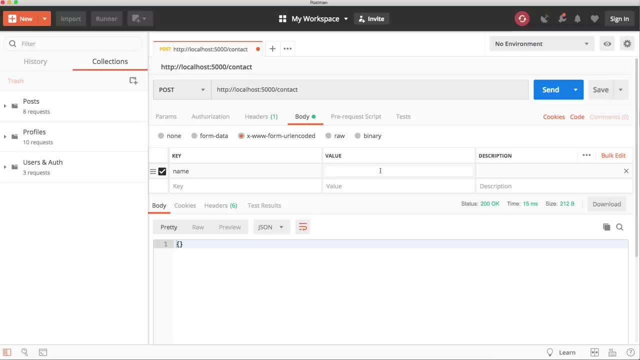 say name. So this is just simulating a form on a website. So we'll say value Brad And let's do a add a city and then add a city to email and Brad at gmail. Okay, so if I go ahead and send, 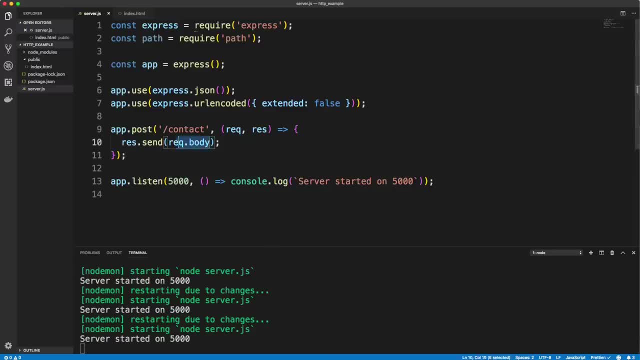 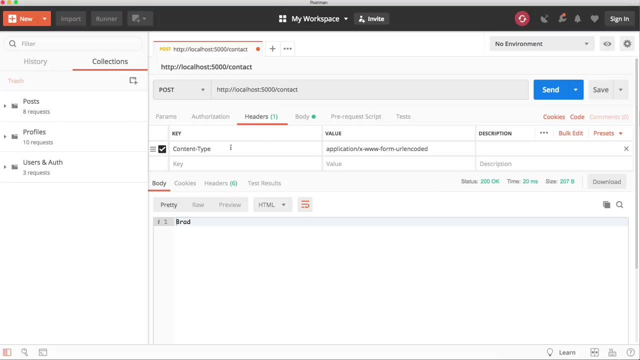 that we're going to see that down here because we sent that we set the request up body. If I do just request dot body, dot name And I send that, we just get Brad. All right, And you see how I sent the content type in the header. If I want to access that, I can do. 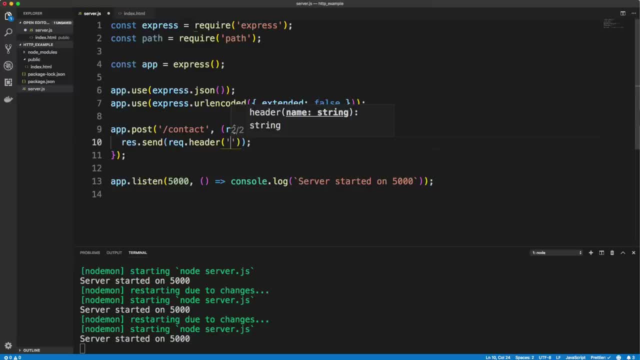 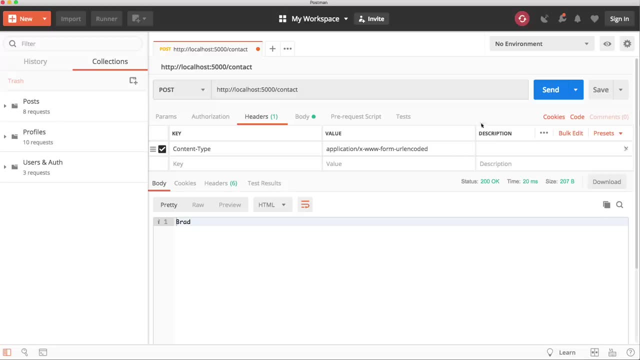 dot header and I can grab the content dash type and let's go back and send and we get this URL encoded. that's the type. alright, we can also send raw Jason. so if I go ahead and get rid of that header and put in a different content type, we 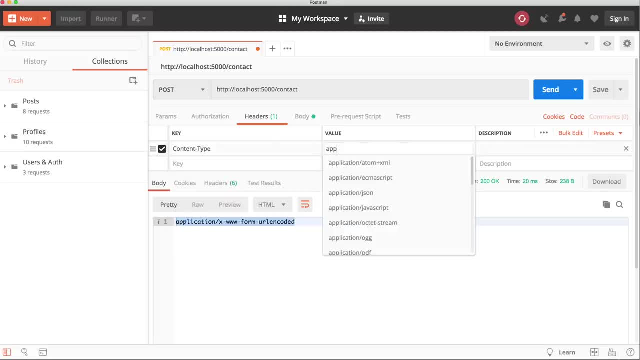 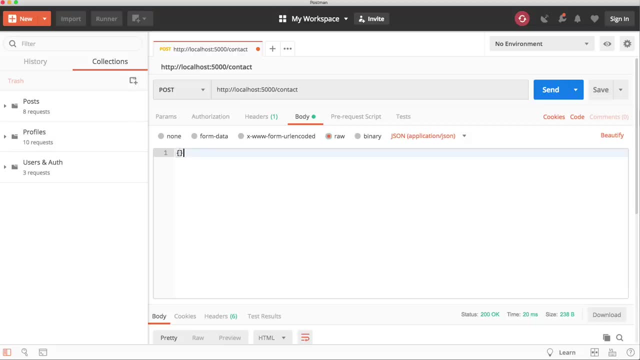 actually get a little drop down here. so content type: I'm going to set it to application: slash Jason, go to body and instead of this URL encoded, I'm going to choose raw- okay, because we can send raw Jason. so name and we'll say John Doe and. 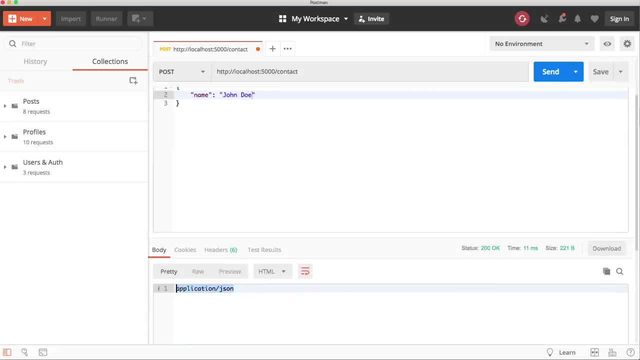 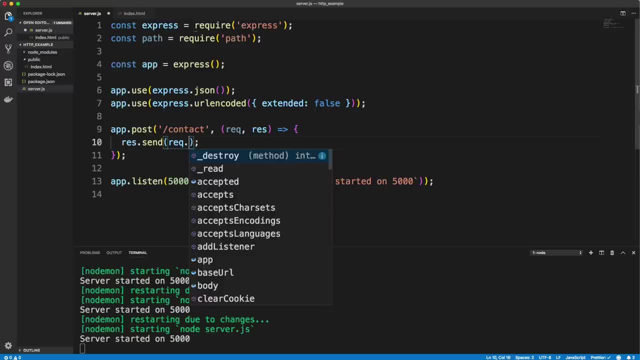 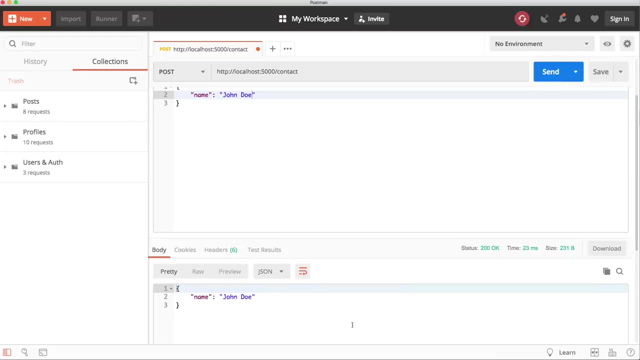 I'll go ahead and send and I get application Jason, because that's the content type, but again, I could access the body if I want. so if I want to get rid of that and just do request body and save and send that, we get our Jason of John Doe, all right, if we look at the 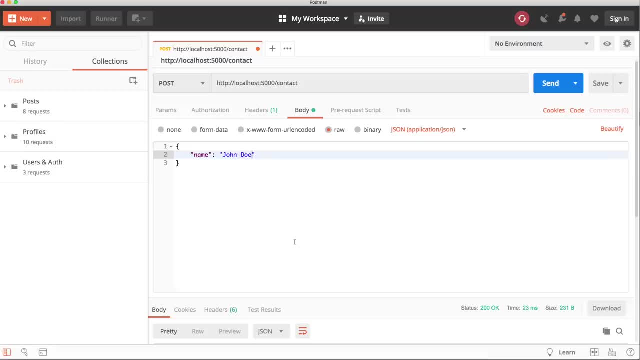 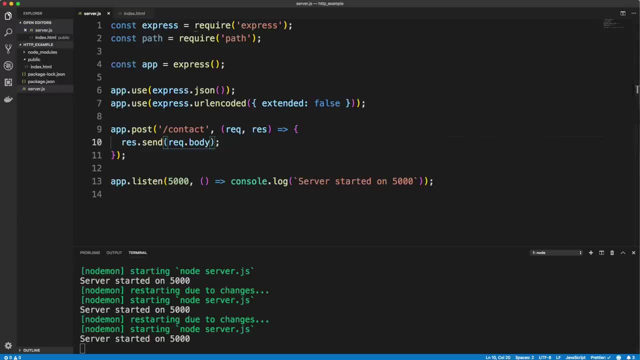 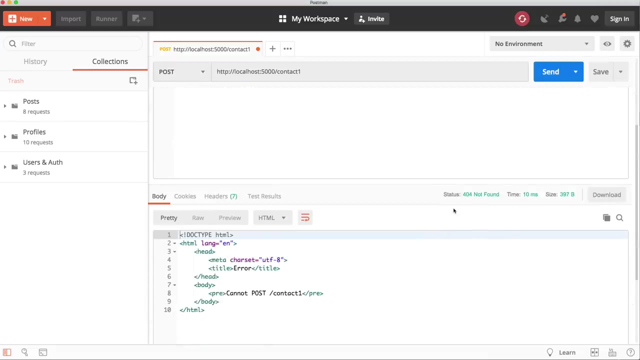 headers, content type. okay, so hopefully this is kind of making sense to you guys that that don't have a lot of experience with this type of thing. now, what about statuses in postman? if I make a post request to contact one and I send that, you can see that I get a status of 404. you guys all know what that means it's. 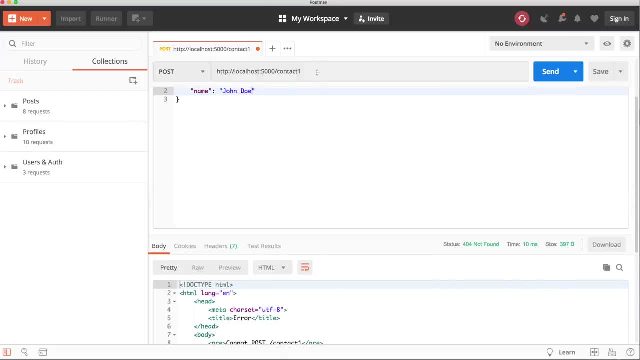 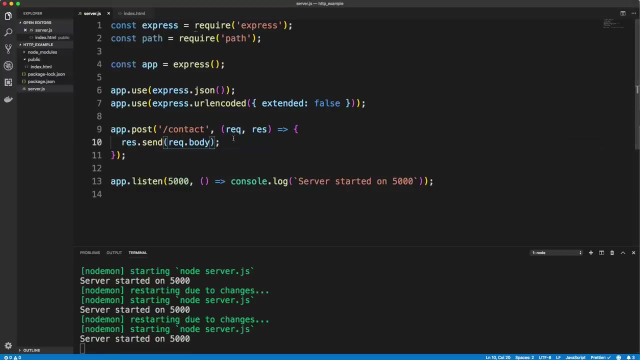 not found me. this cannot post contact one so we can send our own statuses. I mean, when we do a successful rez dot send or rez dot Jason, it's automatically 200, but we can have conditionals and create different statuses based on that. so let's say that: 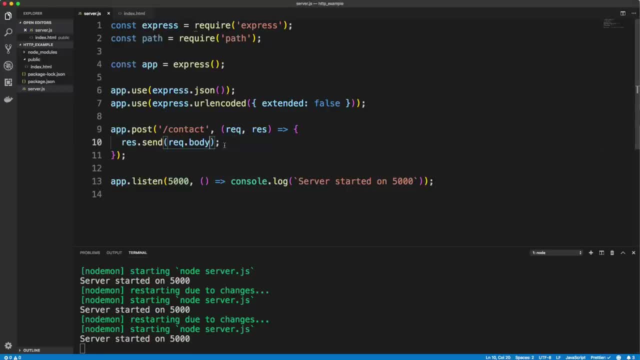 this route. we actually need to have a name. if there's no name, we want to send back a 400 response, which means it's a bad request. so I'll simply do an if statement here and let's say: if no, not request dot, body, dot name, then let's go ahead and do a rez. I'm sorry, want to. 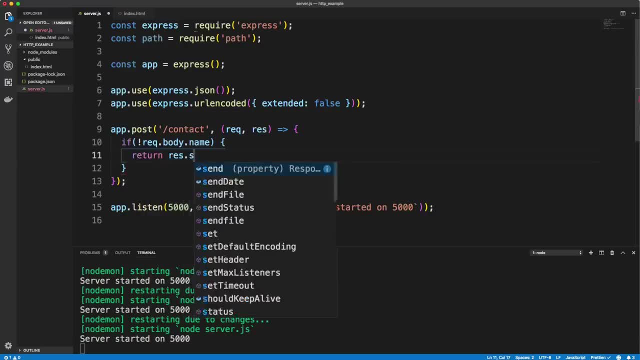 return a rez. dot status cases how we can send a status code. I'm gonna send the 400 and then after that we could do dot Jason or dot send. gonna do dot send and I'm just gonna say name is required. alright, now I'm gonna go under the if statement. 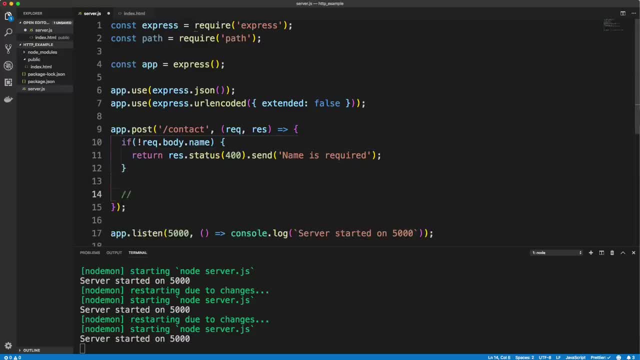 if a name is included, then- and typically you would do like some database stuff here- you would put the, the contact into the database or whatever. but I'm gonna do a rez and I'm gonna do another status here of 201, which means that everything's okay and something was created okay. it means 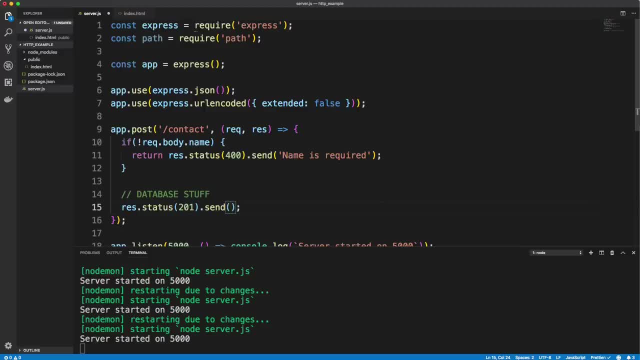 created and I'll do a dot send and then let's just do, I'll put a template string in here and say thank you, and then we can actually put in the request: dot body, dot name. all right, so let's save that. let's go back to postman. 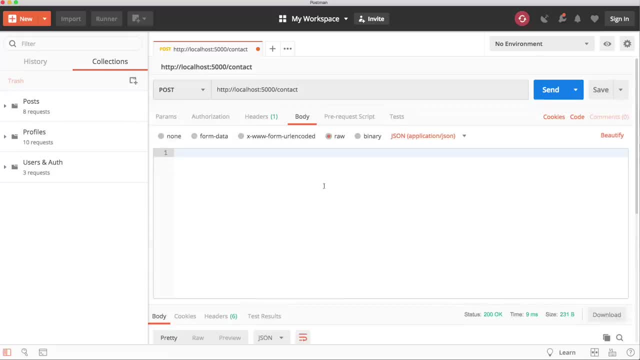 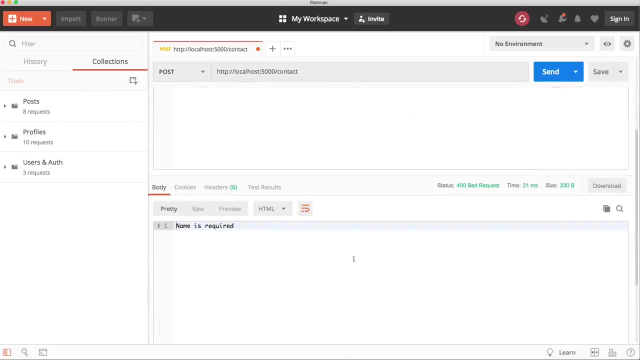 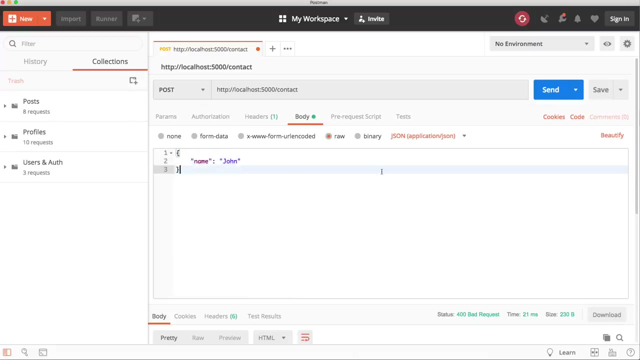 and let's get rid of the name here, let's not send it and we get. name is required, okay, because it's looking for that in the body, in the request body. so if I send it, actually just undo that. so if I say name John and I said now we get. 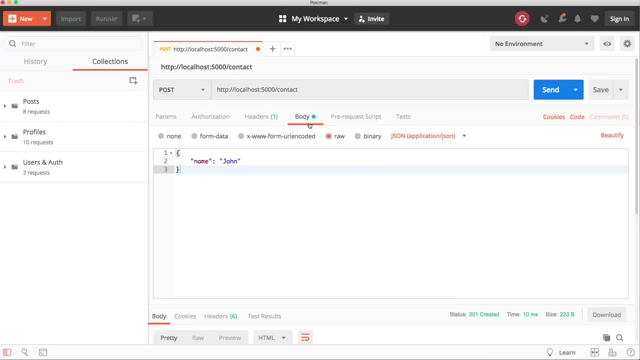 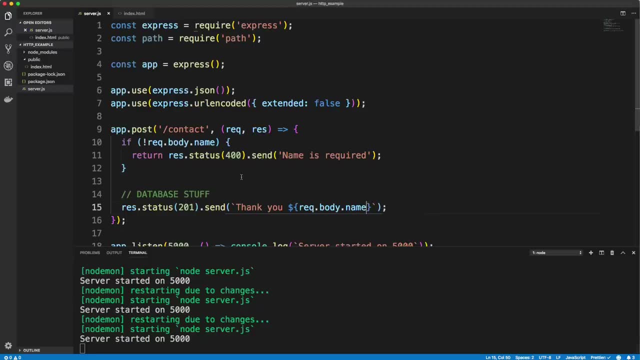 thank you, John, because it passes. we're sending that. that request dot body, that's body name. okay, let's see. so the next thing I want to look at is header values. now, a lot of times when you're dealing with full stack applications, you use tokens or JSON web tokens for for authentication and you send that you can. 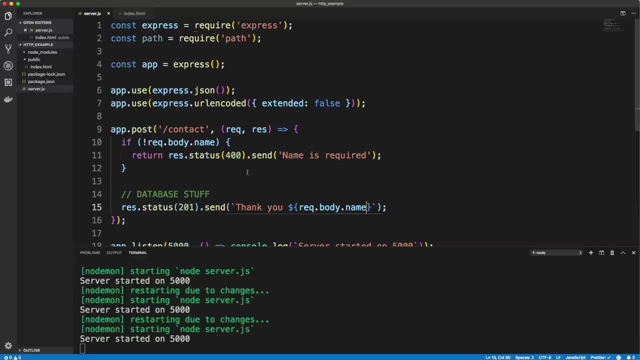 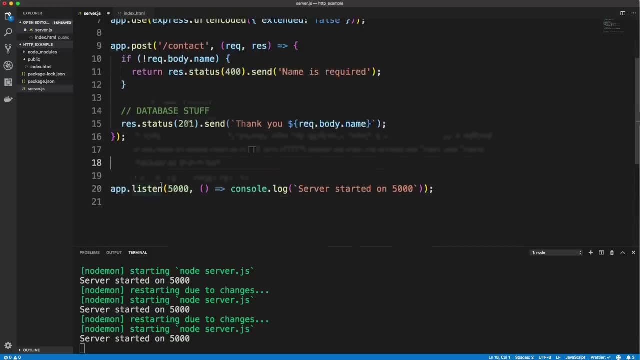 either send it in the authorization. I like to send it in X off token, in a value called X off token. so what I'll do here is create another route. let's do app dot, we'll do post to, let's say, slash login. all right, and then what I want to. 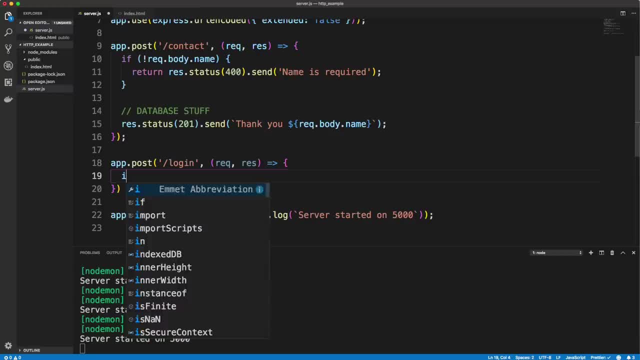 do here is check for a token in the header. so I'm gonna say, if there's no- and then the way that we access header values already showed you this- we can do request dot header and then I'm gonna check for X dash off dash token. okay. so if that's, 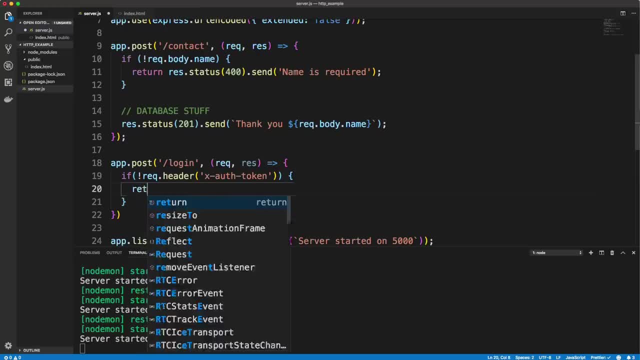 not there, then let's send. let's send an error, let's do return. and one thing I want to mention is notice: I did the return status here and not here. it's because you don't need it if it's the only or the last one, but if you have it. 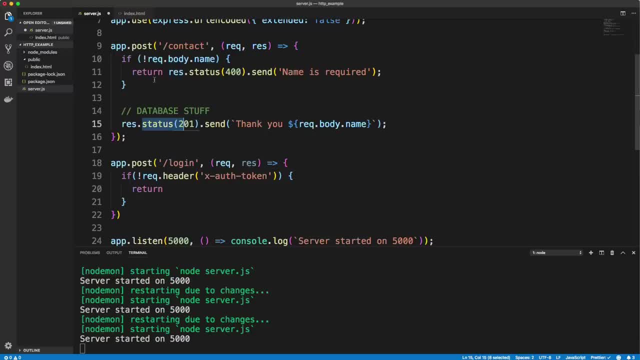 before. if you have another response here, even if it's within an if statement that doesn't pass, you're gonna get an. you're gonna get an if statement that doesn't pass, you're gonna get an error that says headers already sent. so make sure you use return up here, okay, so. 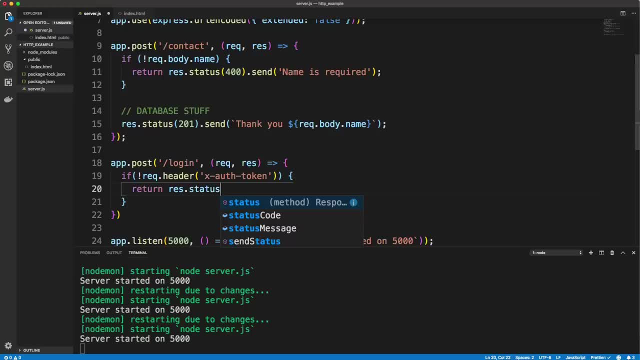 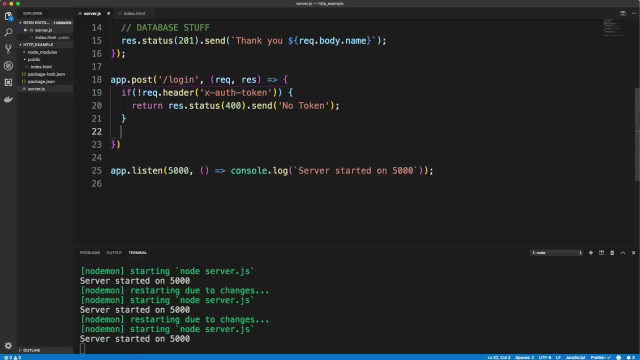 I'm just going to return res dot status and let's say if no token is included in the header, then we'll send a 400 and we'll just send an error that says no token. okay, now let's do a pretend validation for the token, so I'll go. 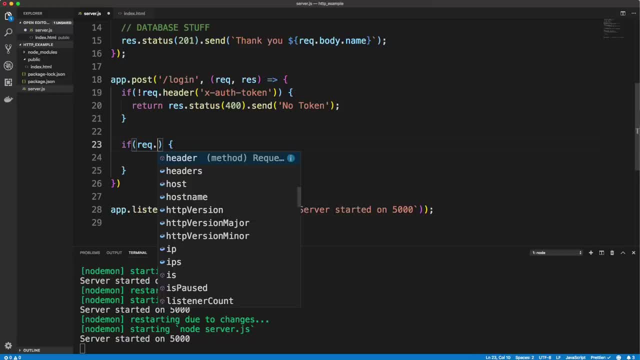 ahead and just say if the request dot header X dash off, dash token, let's say if that is not equal to the string of one, two, three, four, five, six, then it's going to be invalid. so I'm going to return a response status of 401, which is unauthorized. so I'll do send and we'll. 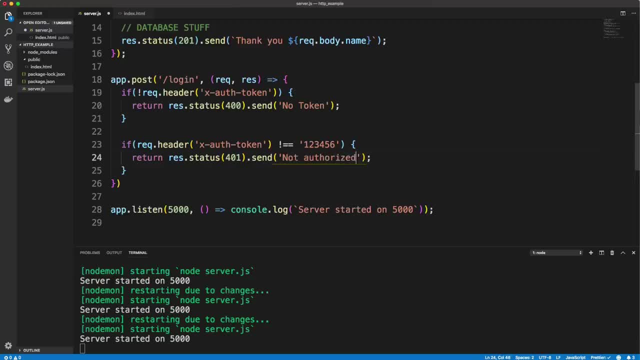 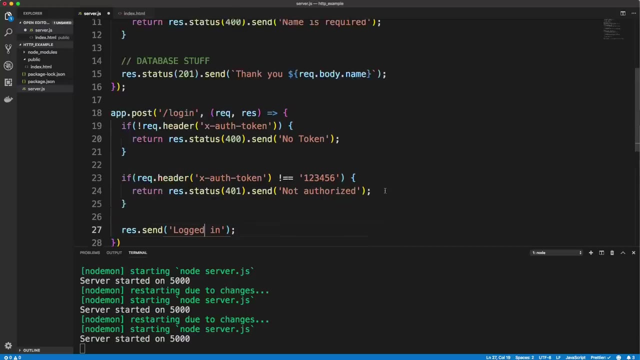 just say not authorized, okay, and then down here, if everything passes, we'll do a res dot send and we'll say logged in. so we're just kind of simulating a login process. obviously it would be much more in-depth. we'd need to use actual token, JSON, web tokens and 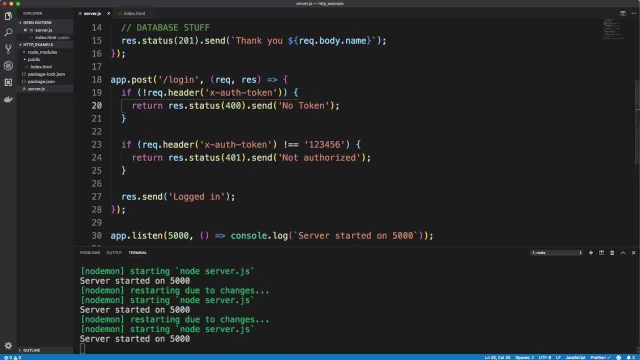 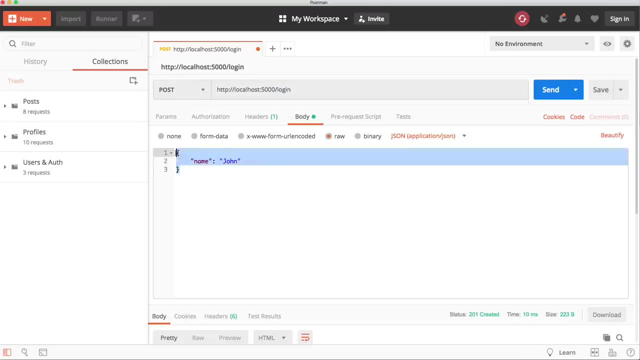 validate them and so on. but let's save that, let's try this out. so if we go back to postman, make a post request to slash login and we don't need any body data because we're just going to go back to postman and we're just going to go back to 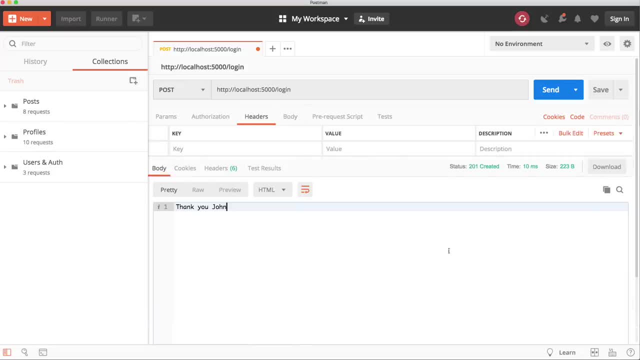 contention. so we're just dealing with headers and we can clear out content type. let's just send that so we get no token. now I'm going to add a header value of x, dash off, dash token, but I'm going to do 1, 2, 3, 4, 5, which is wrong. so 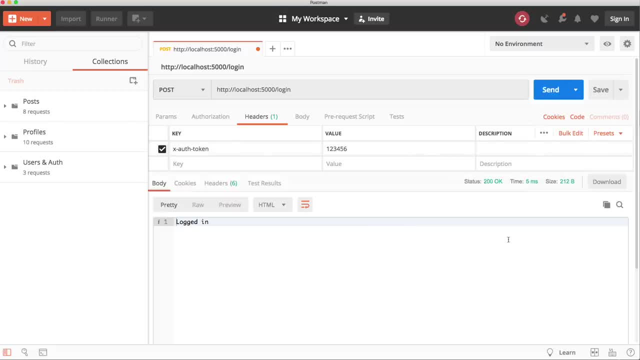 we get not authorized. if I do 1 through 6, we get logged in. okay. so just an example of how you can authenticate through tokens in the in the headers. And, by the way, if you're interested, we do this in my MernStack course. 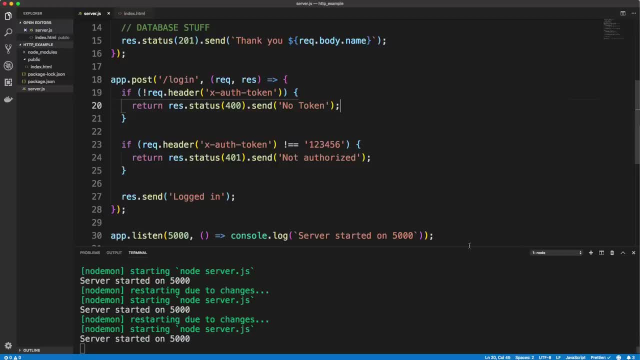 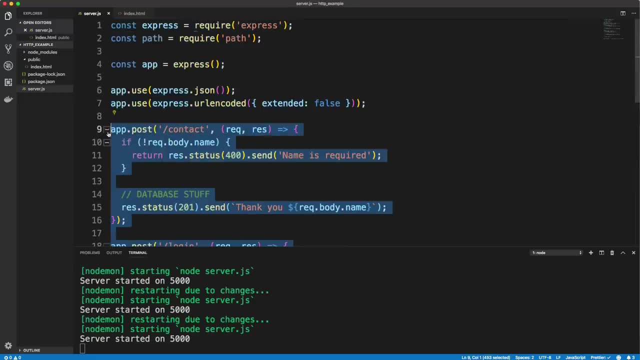 We do all this type of stuff, All right. so let's simulate a put request. So I'm just going to get rid of this. So for a put request we would do appput And maybe it's like a blog post, so we'd have like slash post. 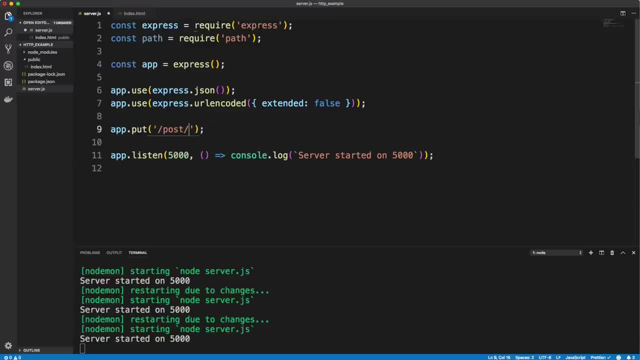 Now, usually you'd have to identify which post you're updating and you would do that within the URL, So it would be like colon ID, which is like a placeholder. All right, and I know that we're doing a lot of express stuff. 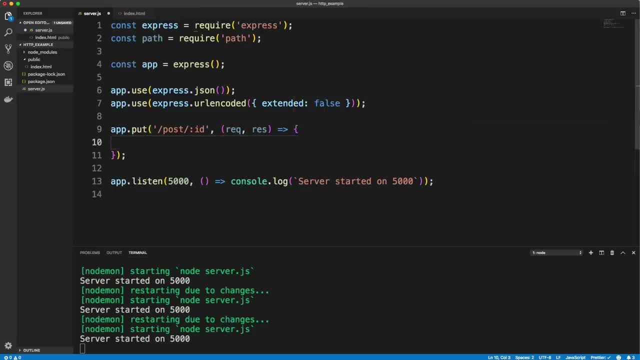 but my goal here is to just get you familiar with sending request, body fields, header fields, dealing with that, sending status codes back. So here usually what would happen is we would do some database stuff- Oops, So database stuff- to update the post and then send back a response. 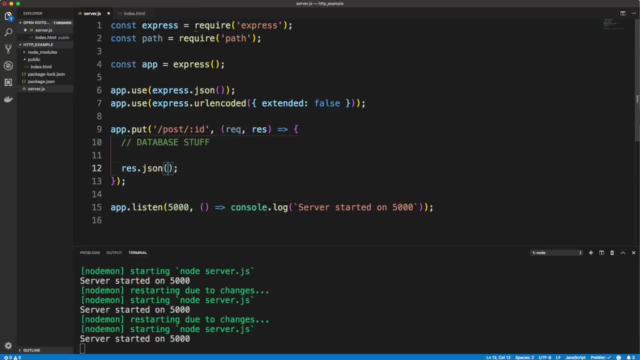 Let's do a resjson And we'll send the ID. Now, if you want to get the ID that's passed in, you can actually use requestparams and then whatever the param- in this case ID- And then the title we're going to send in the body. so I'll do requestbodytitle. 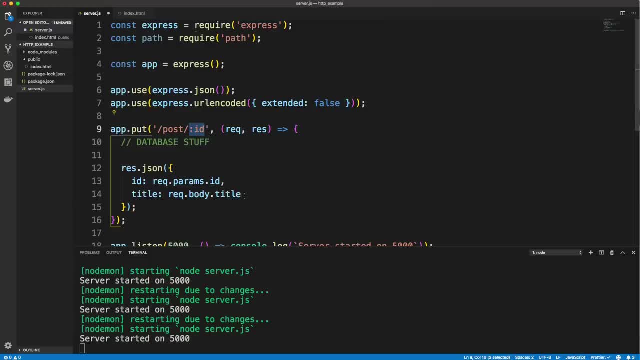 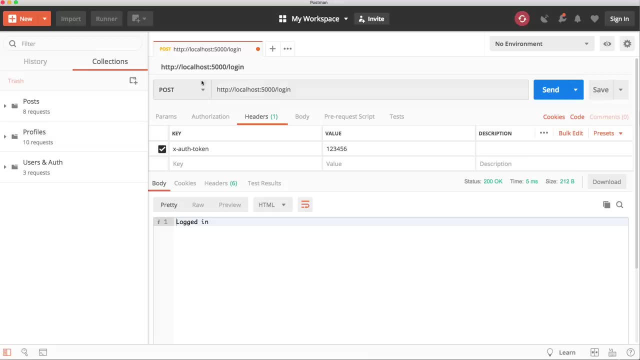 Okay, so requestparams is going to access the URL values. Requestbody will access the form data or the JSON data that you send in the body. So we'll save that and from Postman we can make a put request to slash. 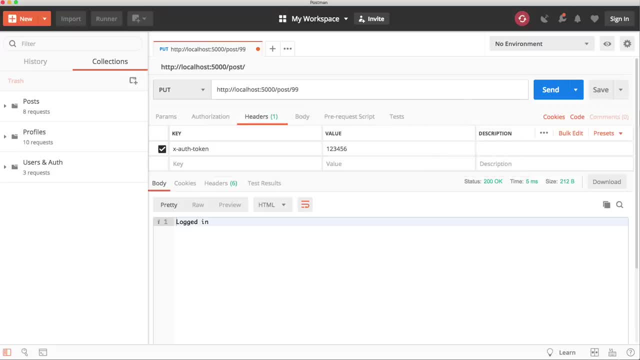 and we'll do post slash 99.. Okay, so this will get accessed with requestparams and then in the body, since we're going to be sending data, we actually have to add a header value of content type, And I'm just going to send raw JSON, so we'll do applicationjson. 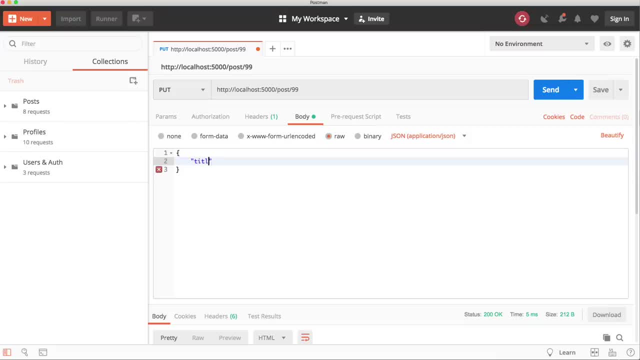 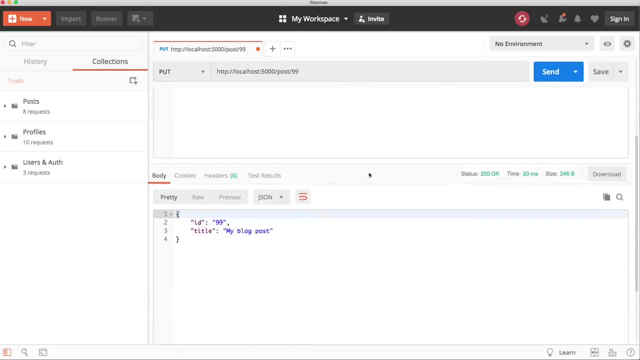 and then let's send the title- So title my blog post. And if we send, we get a response back with the ID of 99, because that's what we put in here- and then the title: that's what we put in the body. 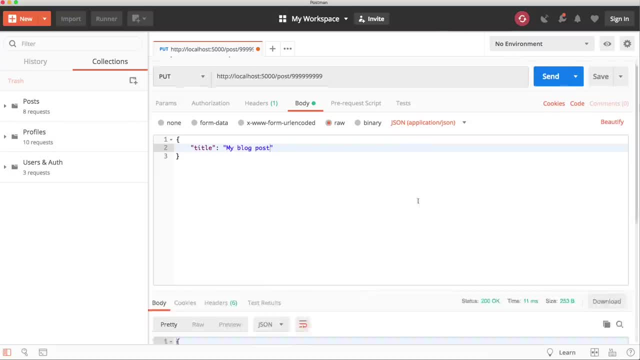 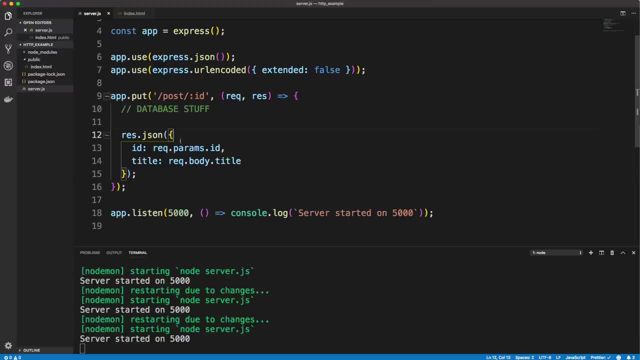 And I could put anything at all in here. Okay, so hopefully that just gives you an idea of how put requests work. But typically you would do an update of the database using that ID And then delete would basically be the same thing. 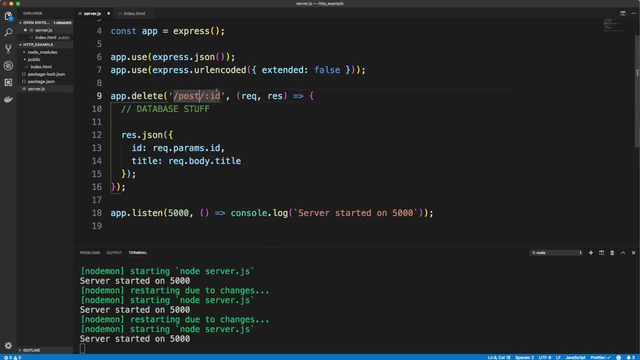 So we just do appdelete and include the ID, delete it in the database and then return, maybe most likely not going to return the post because it's deleted, so you might do something like a message message and say post. Actually, what we could do is 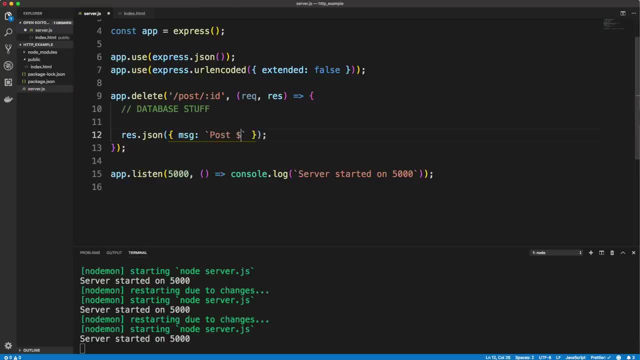 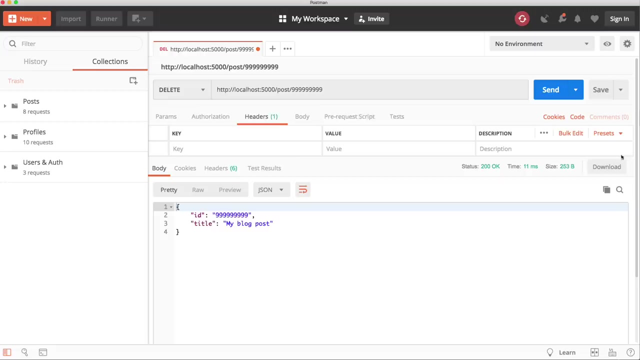 we could say post and then take the ID and say deleted. Okay, so now for postman, we could make a delete request. We don't need any of this. We don't need this in the headers. We could just send that. we get post that deleted. 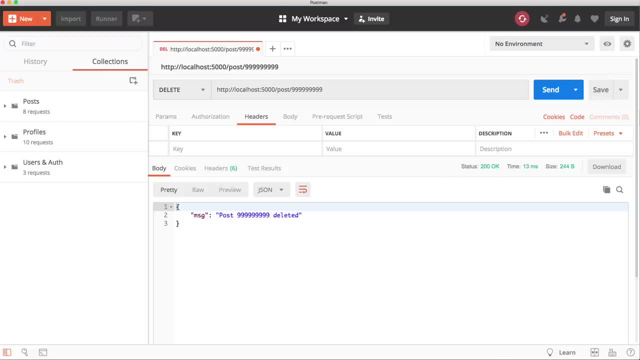 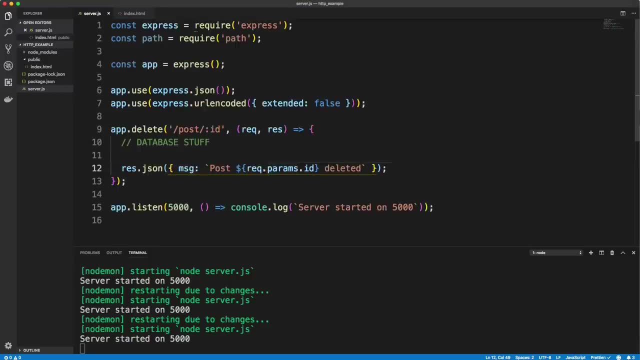 All right. so yeah, I mean, hopefully this helps a little bit Understand how this goes. now, with express, We can set a static folder and this pertains to if you just have a static HTML website. we have a bunch of CSS files and JavaScript files and stuff like that. 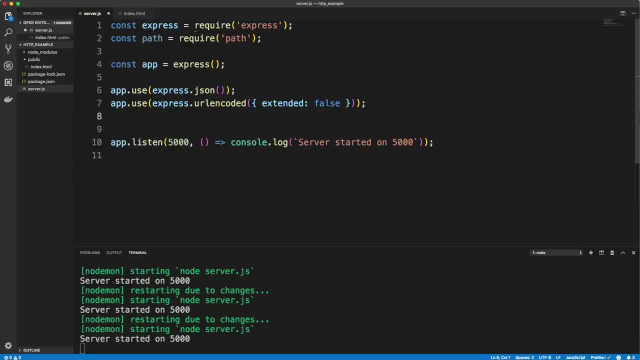 So in express what we can do is we can actually set a specific folder to be our static folder, And we do that with appuse And in here I can just say expressstatic, And then in here I can put the location of the folder. 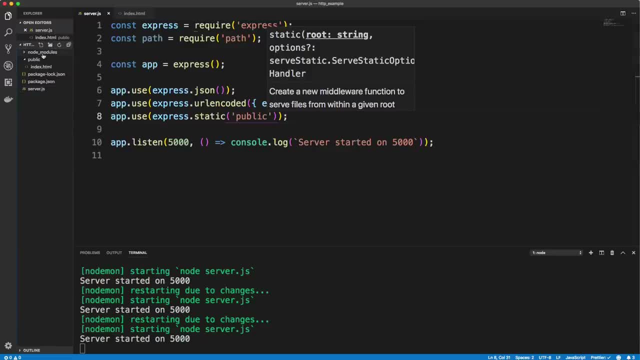 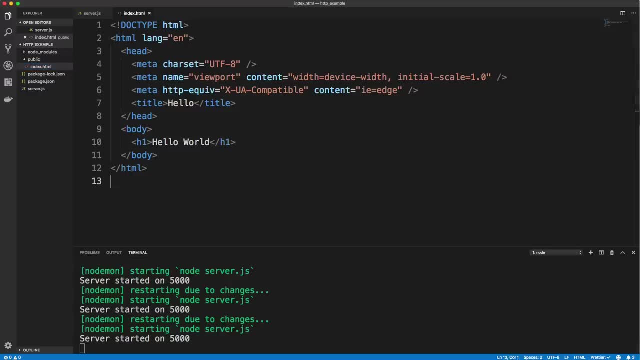 which is gonna just be public. So now in my folder structure actually I already have a public folder. I forgot. I created that with an index HTML file that just says hello world. So I should be able, even though I don't have a route. 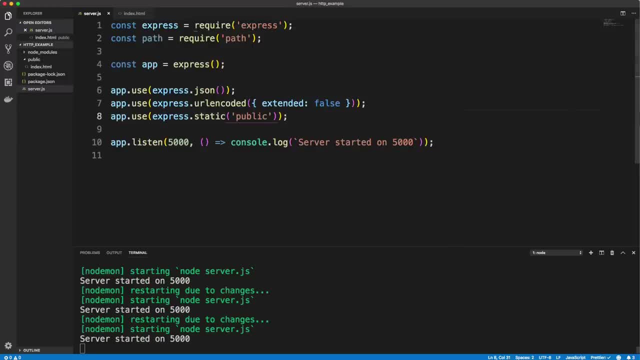 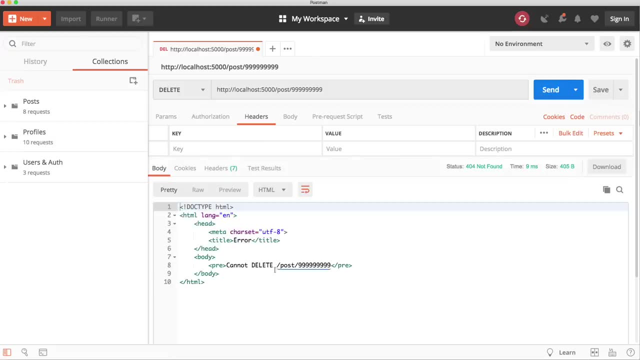 for my index page. I have this static folder So that should load the HTML file. If I go to my browser, we can see it there, And if I go to postman we can see. oops, we wanna make get. 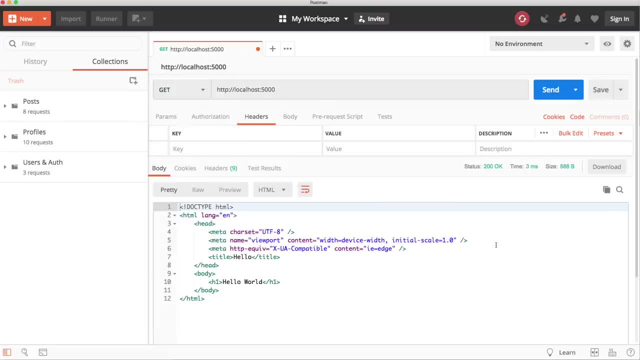 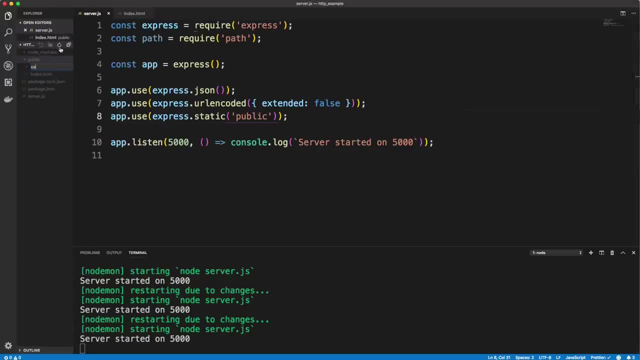 To the index and now we can see the hello world. If I wanted to create some CSS files in my public folder, I could do CSS and create stylecss and we'll just do body. I'll say background: sky blue. So I'll save that. 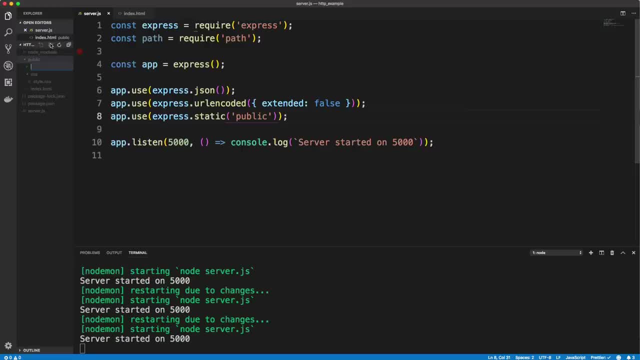 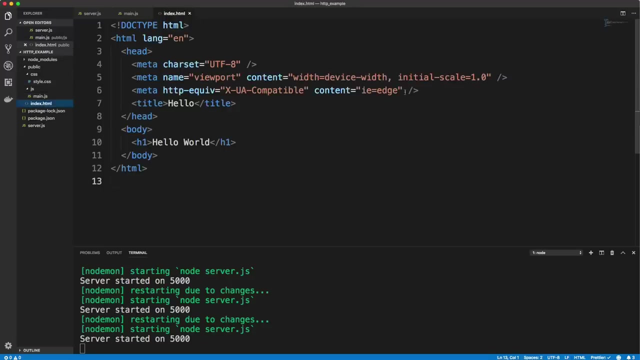 Let's create a JavaScript in our public folder as well. We'll say folderjs And file mainjs And I'll just do a console log of one, two, three. I just wanna include these files in my HTML, So back in my HTML I'll do a link to CSS slash style. 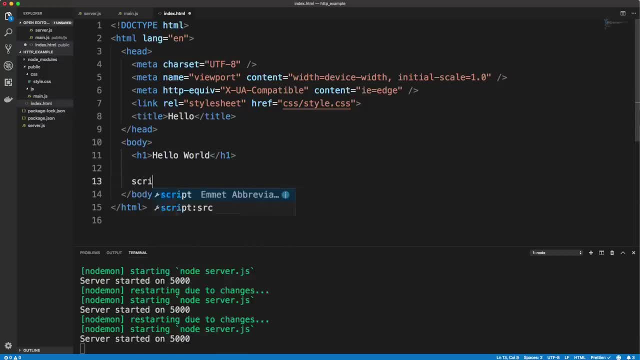 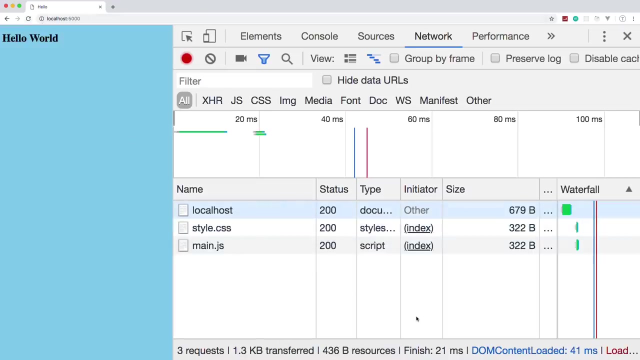 and then I'll link my JavaScript down here: Oops script source and js slash mainjs. All right, so I just wanna show you that if I go to Chrome now and I reload in my network tab, I'm gonna see all those files. okay.